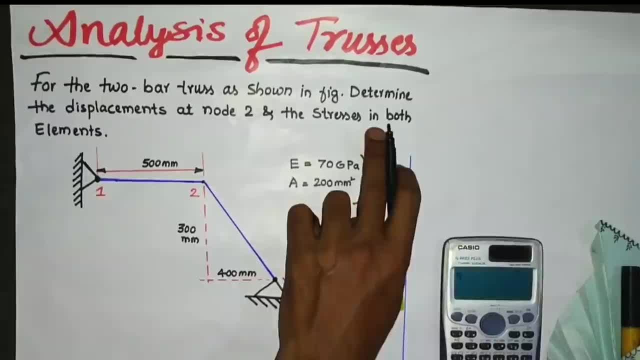 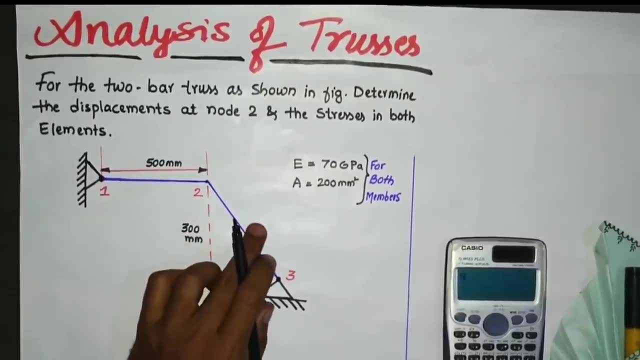 to be calculate. and also you need to calculate the stress in both the elements. So you need to calculate the stress at the element 2.. So you need to calculate the stress at the element 2. And also stresses in the element 2. We have to calculate. So in the truss element the concept. 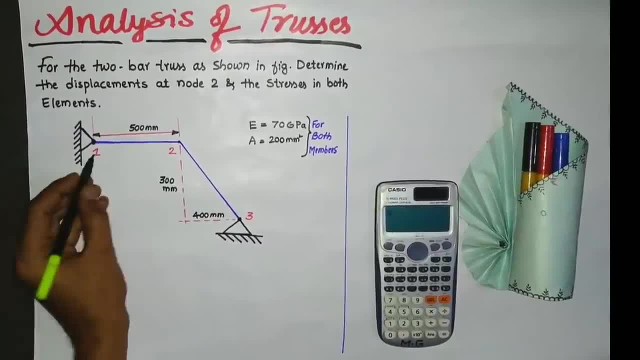 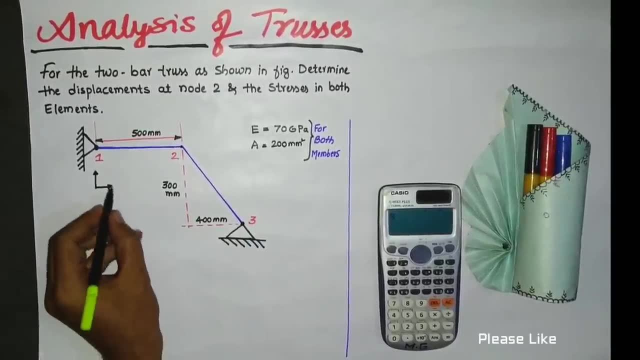 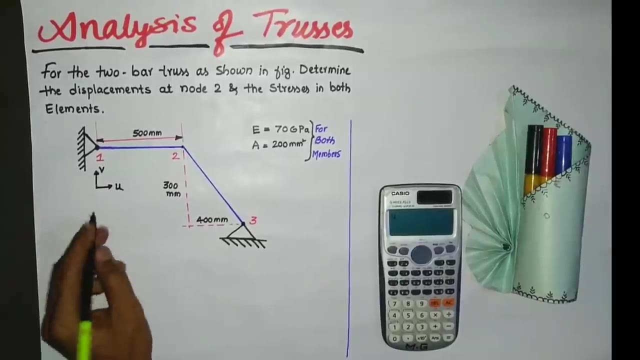 is that at each node you will have the two displacement. Suppose, at the node 1, we will have the one horizontal displacement, another vertical displacement. So we will represent the horizontal displacement with u and whereas vertical we will represent with v. So at the node 1, it will be u. 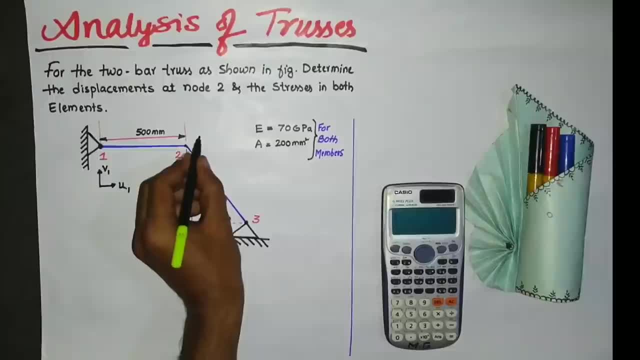 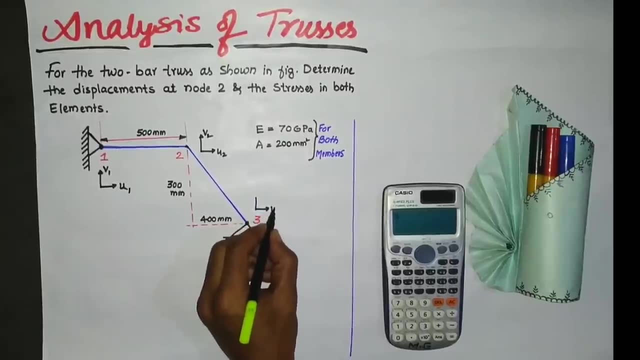 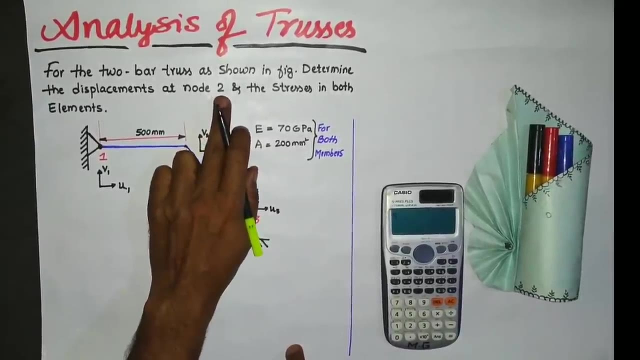 1 and v1.. Similarly, we will represent at 2, u2, v2 and at 3, it will be u3, v3.. So these are the displacement. Now you are calculating. the displacement at 2 means you are calculating u2. 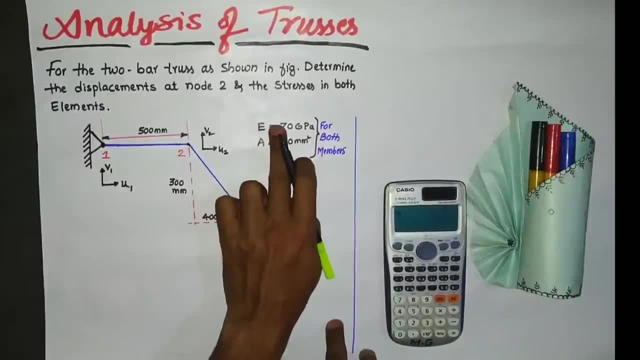 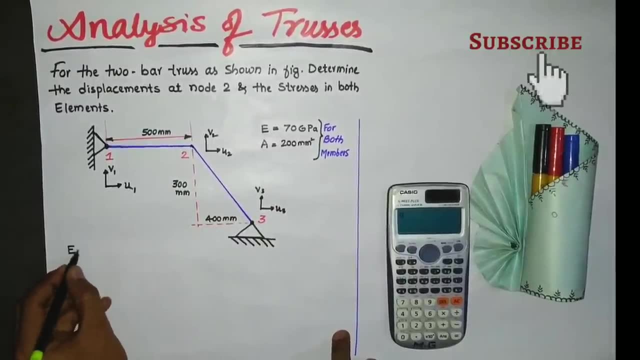 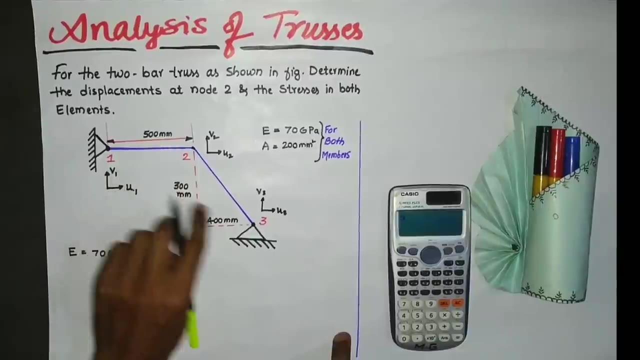 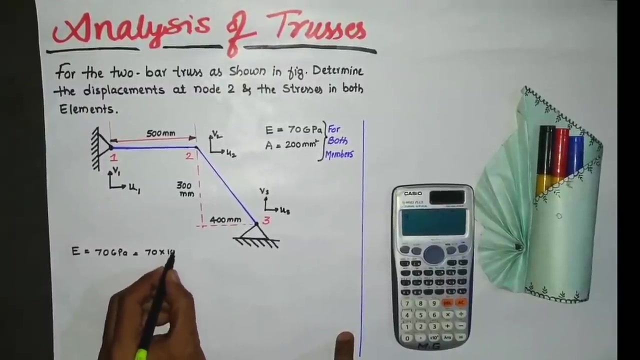 and v2.. And the material properties, like Young's modulus is given that is 70 gigapascal, So that E is equal to 70 gigapascal. So here all the units are in millimeter. the length, some other dimension, are millimeters. So convert that Young's modulus is also in millimeters, So 70 into 10. 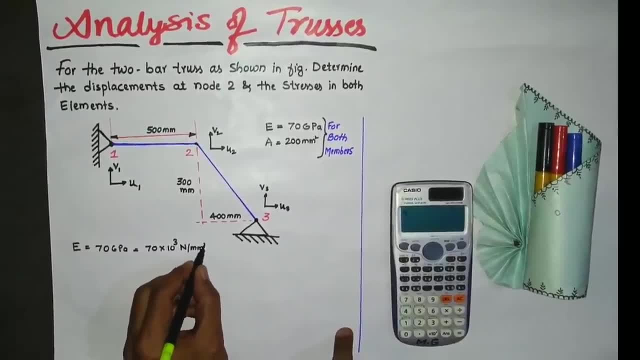 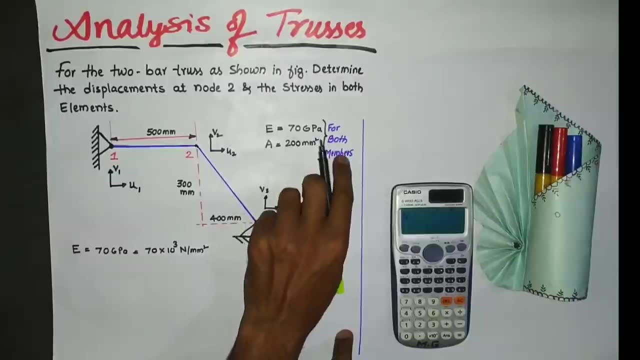 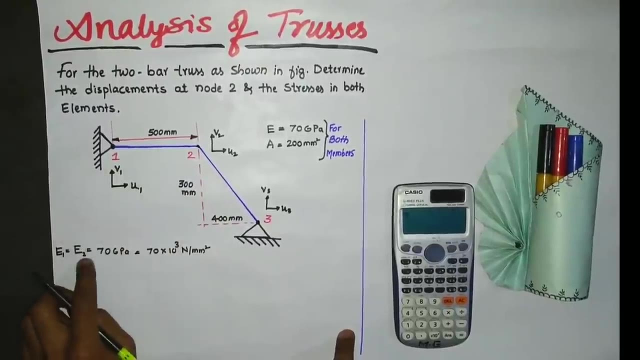 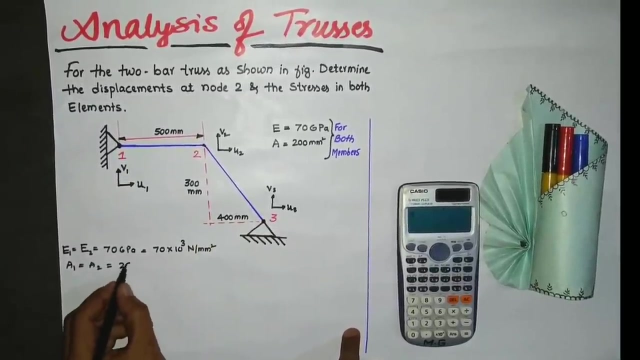 power of 3 Newton per millimeter square. Next, the area of each material is 200. for both the members means for E1 is equal to E2.. We have two elements, So E1, E2 and also area A1, A2 is equal to 200. 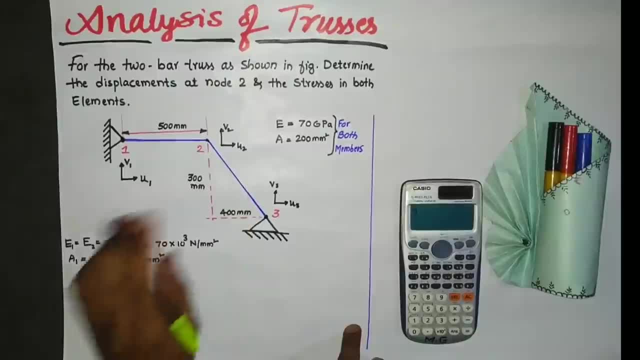 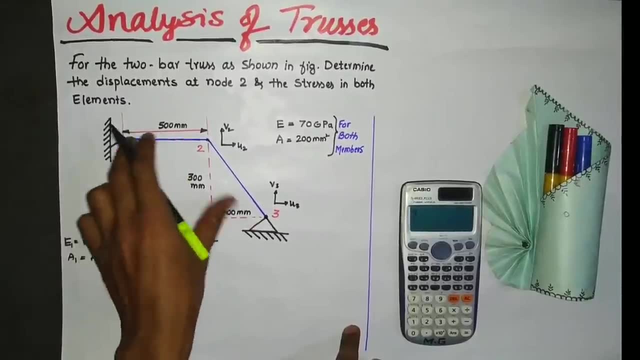 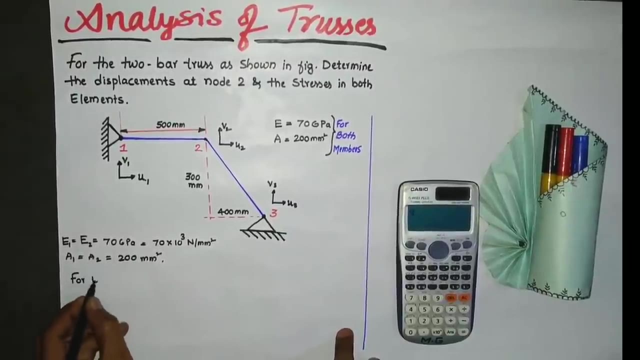 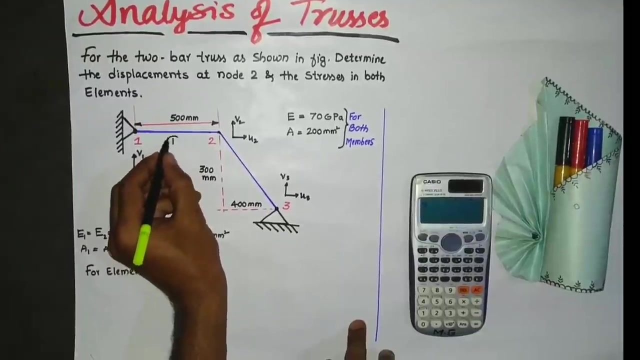 millimeters square for both the elements. Okay, so once you have made all the given data, then we'll go for calculating the element stiffness matrix for the truss. So suppose for element 1.. So let us take this is as element 1 and this is as element 2, we can represent. 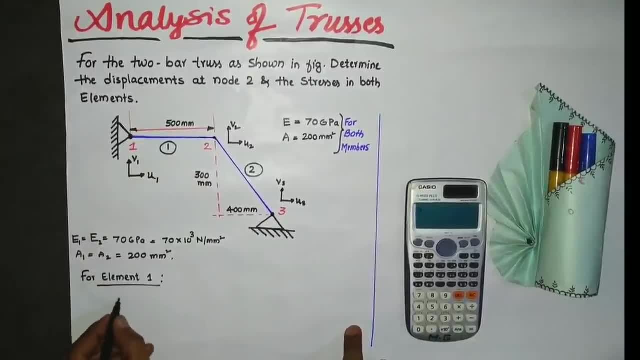 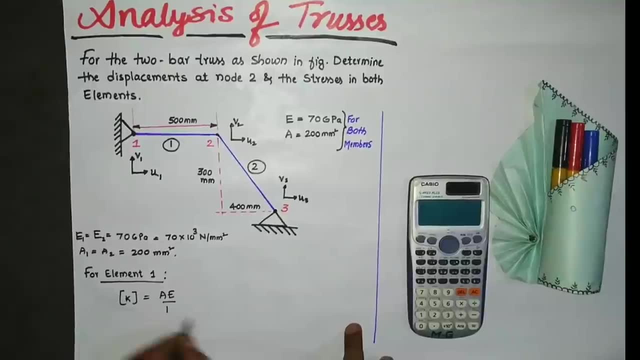 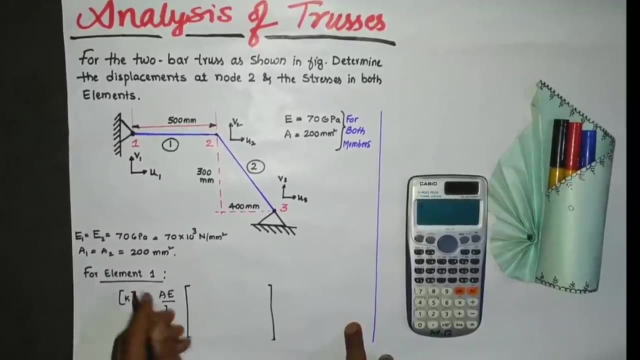 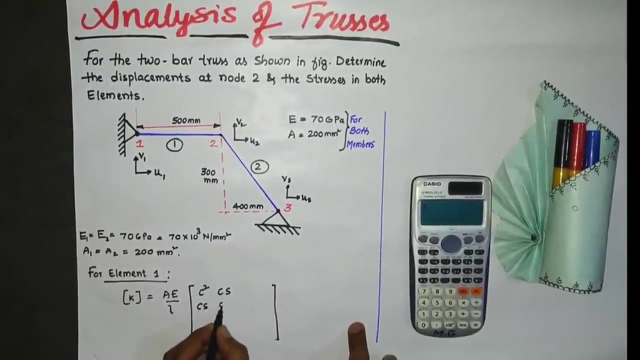 So at the element 1, you need to calculate the stiffness matrix, So K is equal to AE by L. For element 2, we need to calculate the stiffness matrix, So K is equal to K by L. So this is a 4x4 matrix. for the truss element It is C square, Cs, Cs, S square. 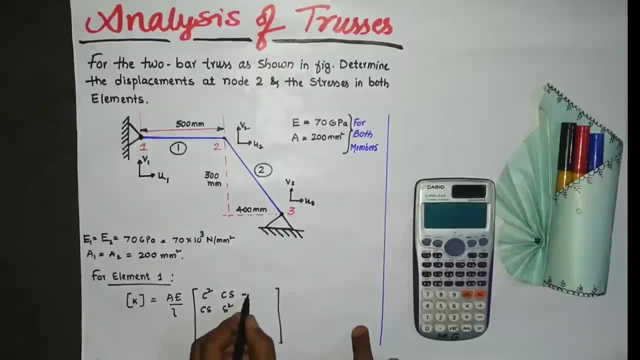 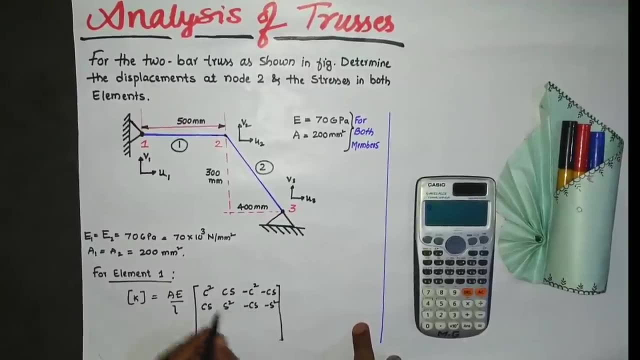 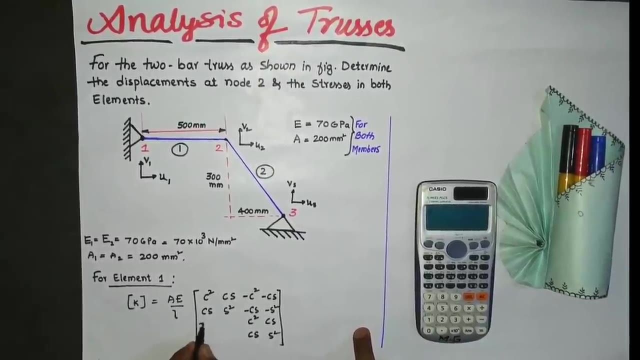 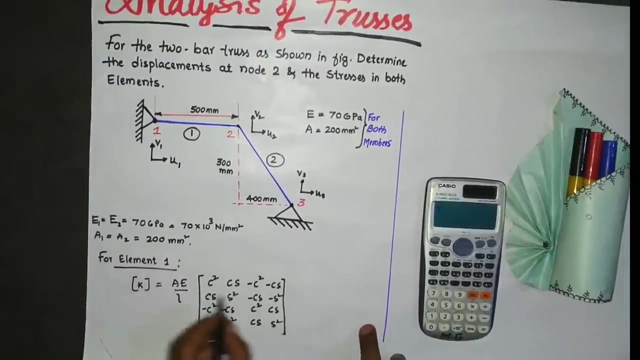 So it is an asymmetric matrix. So here it will be in the diagonal minus C square, minus Cs, minus Cs minus S square. So diagonal it should be same C square, Cs s square, minus c square, minus c s, minus c s s square. okay, so sum of the textbook it will be. 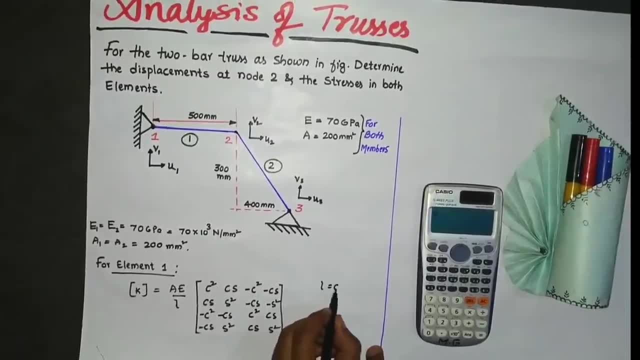 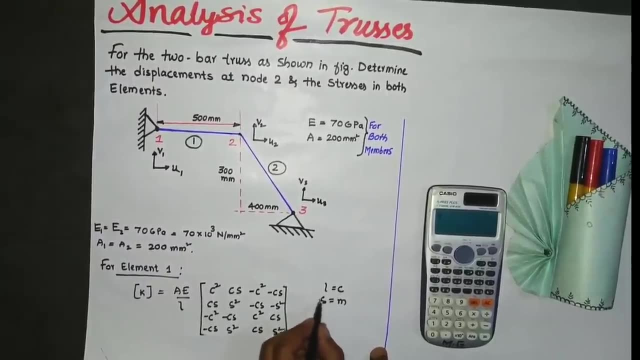 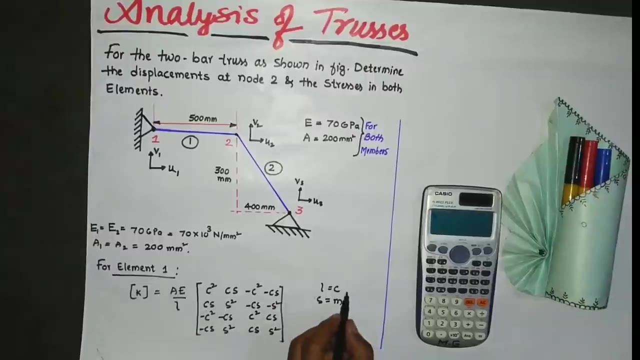 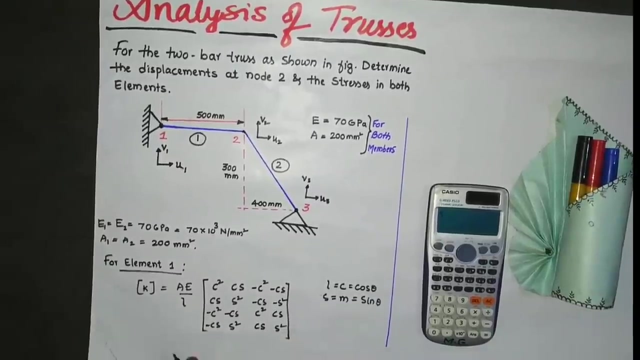 represent with l as c and s as m. okay, so l as c, and where m as s, it will be represented. so now you should know what is c. so c is nothing, but it is an, a cos theta, where s is nothing but sine theta. and first we will calculate the a by l. so, area of the element, one angst modulus for the. 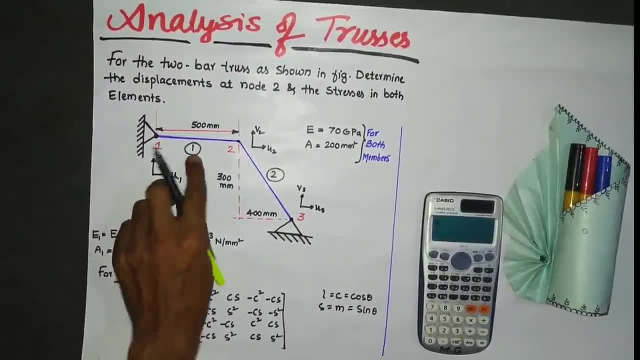 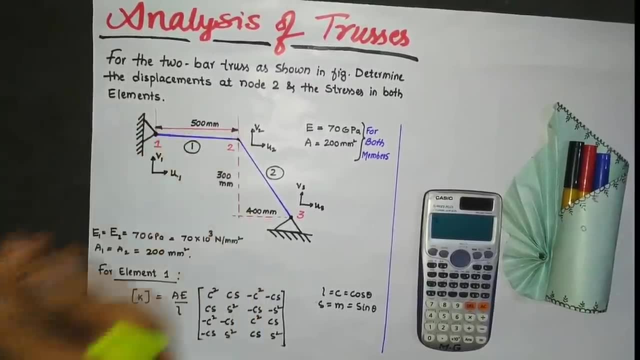 element one divided by the length of the element one. so for the element one we know the length is 500, so that length is directly given in the question. so that is 500. so first we will calculate the length of the element one and then we will calculate the length of the element one. 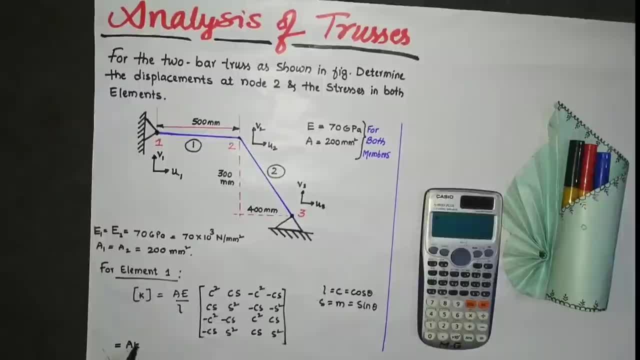 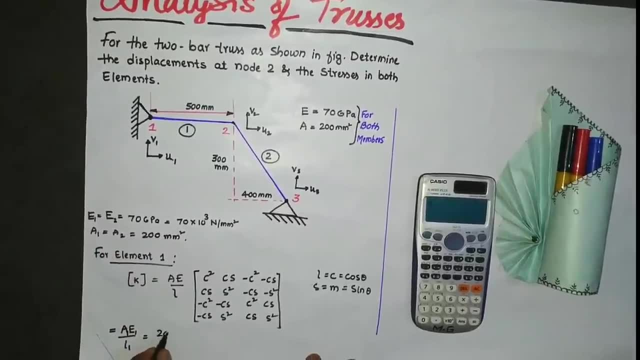 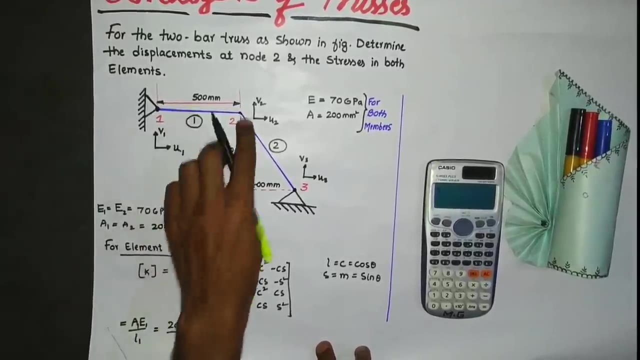 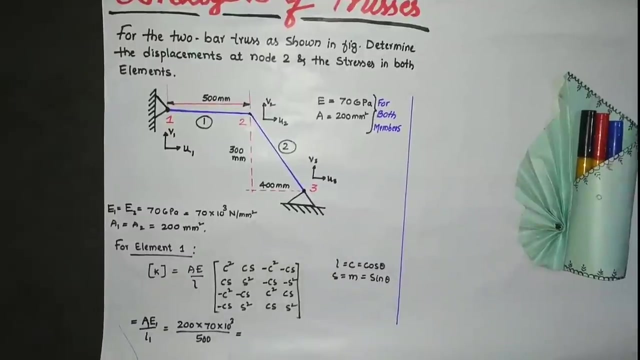 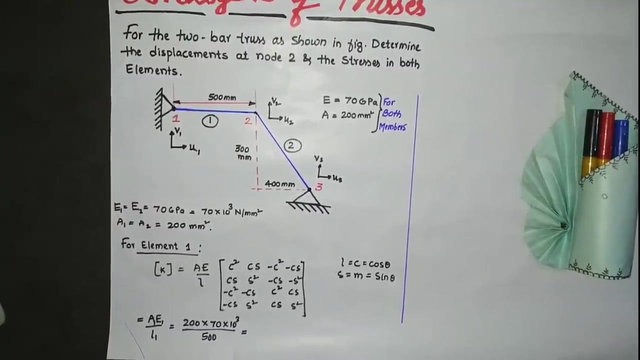 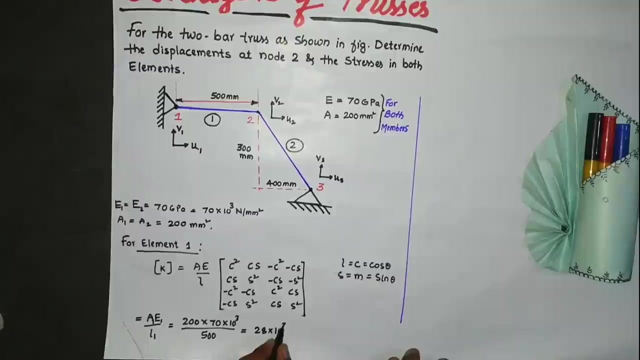 for the element one: a, e by l, a1, e1 by l1, so a1 is 200 into e1, 70 into 10. power of 3 divided by the length. for the element one is 500, so i got 28 into 10 power of 3 newton per millimeter. okay. 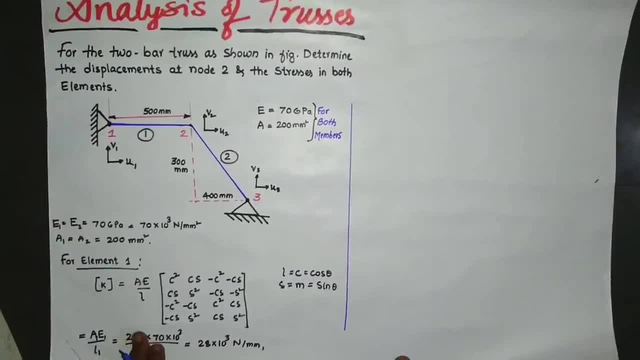 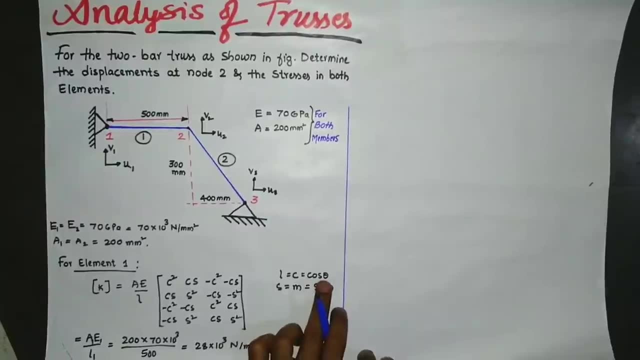 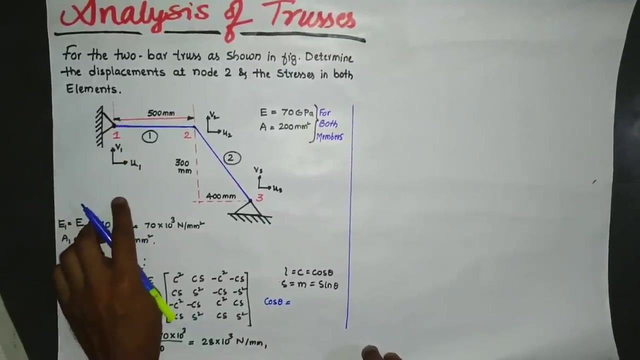 so after calculating the a by l, so we will calculate the c and s value. so c is nothing but cos theta. so cos theta we can calculate from the geometry, or also by making the geometry in the coordinate system we can calculate the angle cos theta and sine theta. 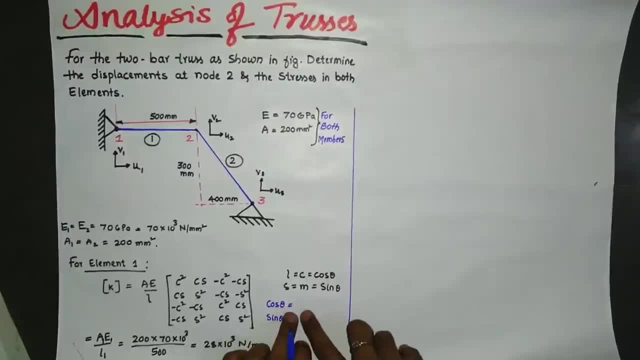 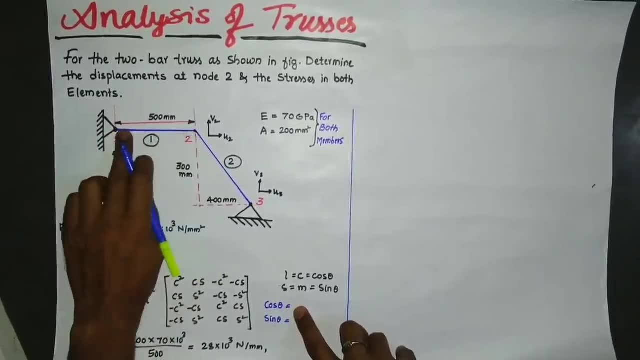 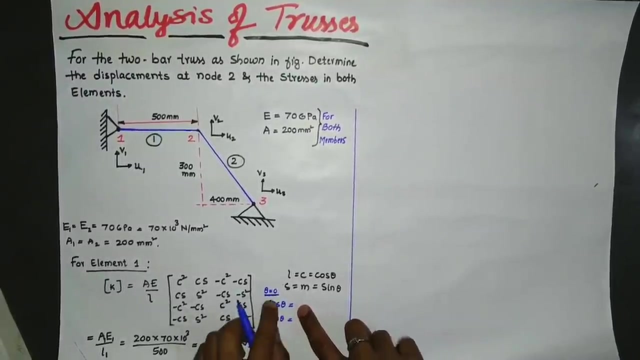 so suppose, if you want to calculate by the geometry, so from the geometry for the element one, it is at an angle of zero degree where theta it will be zero degree. that is the one case. so in one method we can calculate like this: so the theta is zero degree, so cos zero degree it will be. 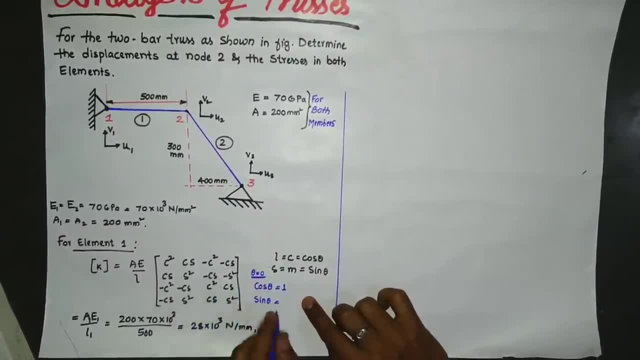 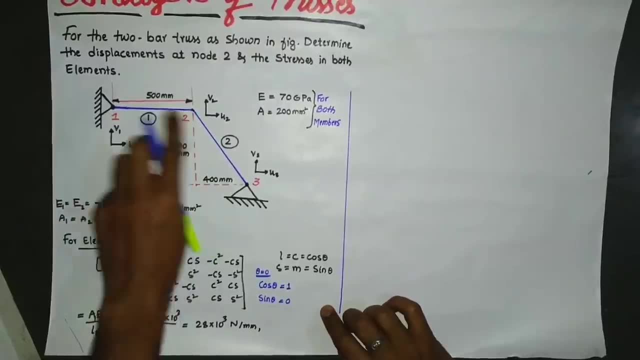 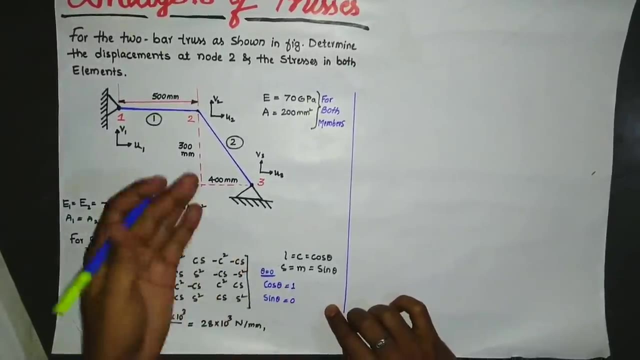 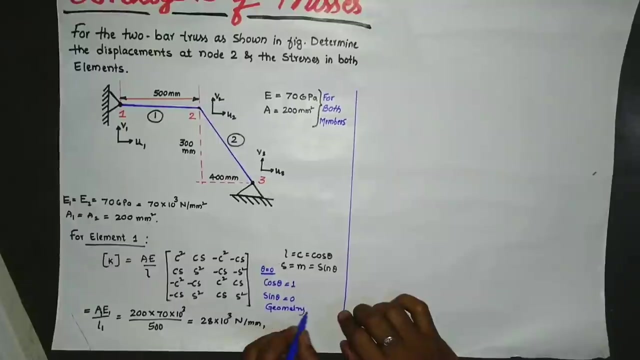 one, whereas sin zero degree, it will be zero. okay, so like that, directly you can take when, in case of a zero degree, or if it is an perpendicular angle, we can easily calculate the cos, theta and sine theta. and the second simple method is to take from the geometry, so by the geometry, so here: 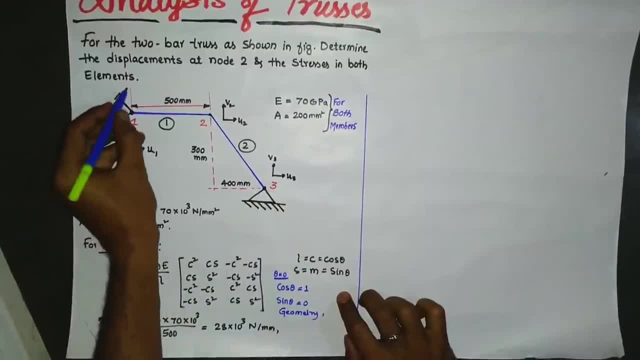 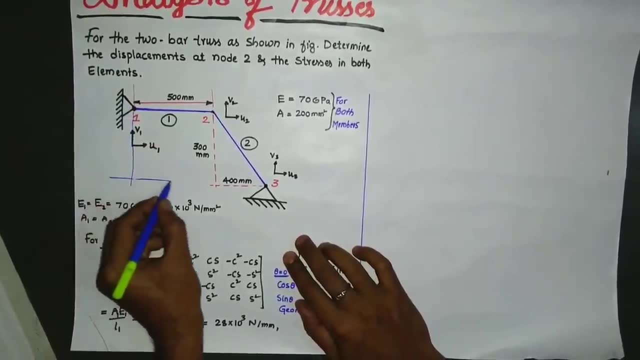 the entire truss element. it can be calculated by the geometry and sin theta and cos theta can be located in any one of the quadrant system. suppose, make this as in the one quadrant system. so i am taking the entire system in a first quadrant so this become in the first. 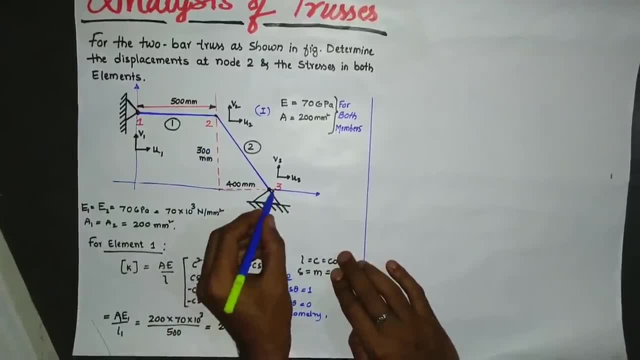 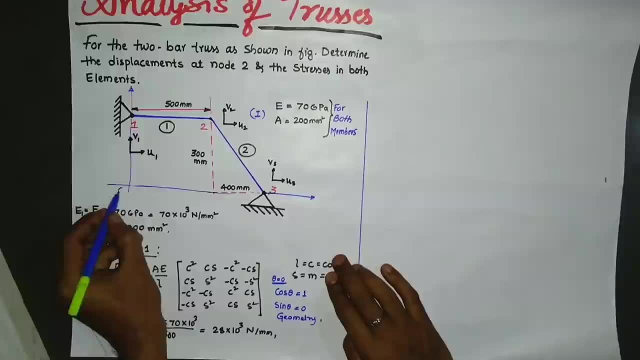 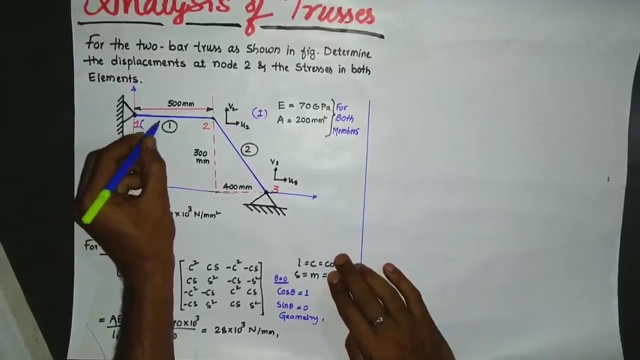 quadrant. okay, so where one node, it should touch us with the horizontal line and another node should touch with the vertical reference line. so here it will be 0. now from the reference line you have to find out the coordinates at each nodes. so here at the node one, so what? 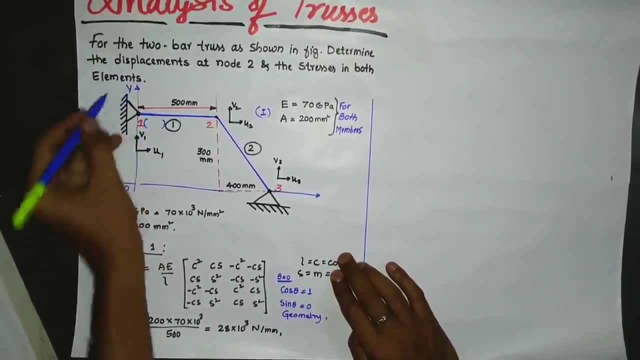 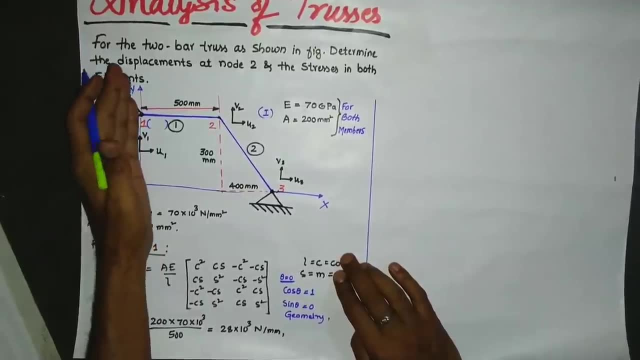 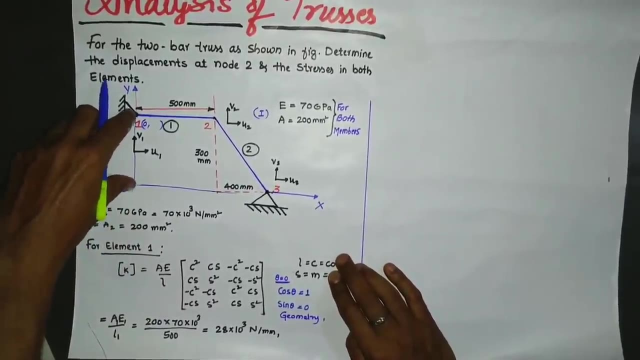 is the x distance from the reference line o y and this is o x from the reference line o y to the that node. so where x is 0 and y distance, it will be the height. so this height will be the y distance. so that is 300.. 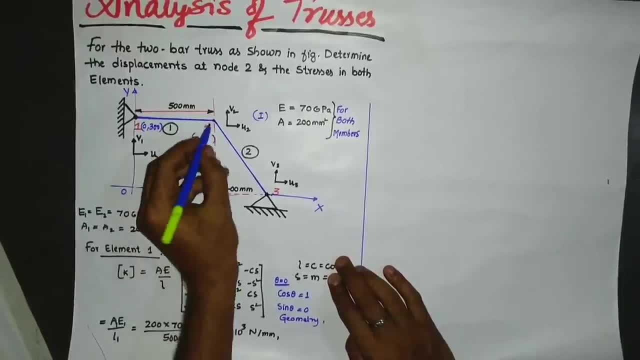 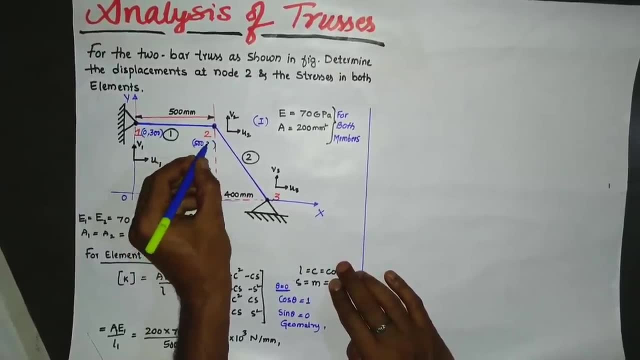 similarly, if you want to find out the coordinates at each node, then you have to find out the coordinates at each node. so here at node two, so at node two we have the node here. so x distance it will be 500 and y is 300. from the reference line o x to this height is 300. 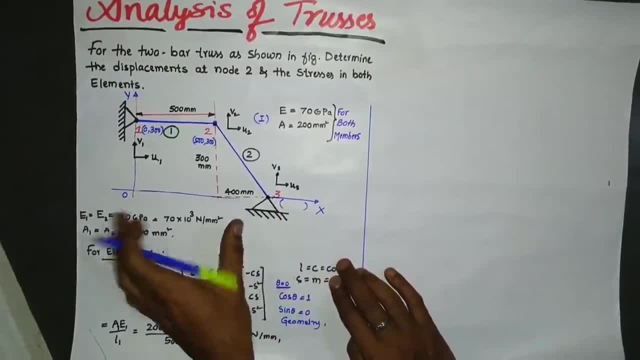 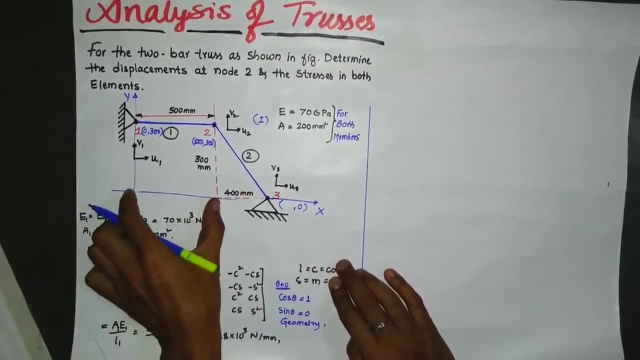 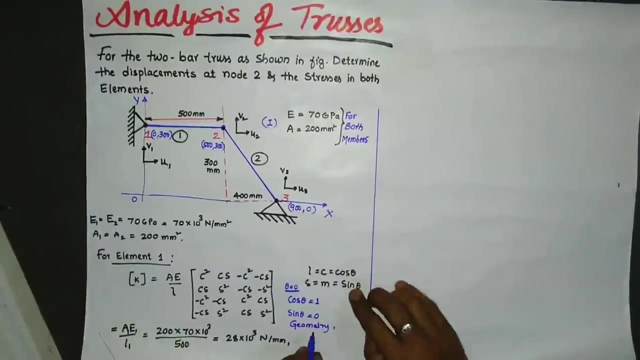 now come to the node three. so at node three this is x distance and y it is on the reference line. so y is 0 and x. this distance is 500 plus 400. so totally it will be the x distance. it is 900 now. so for the element one, now we are discussing with only element one. so 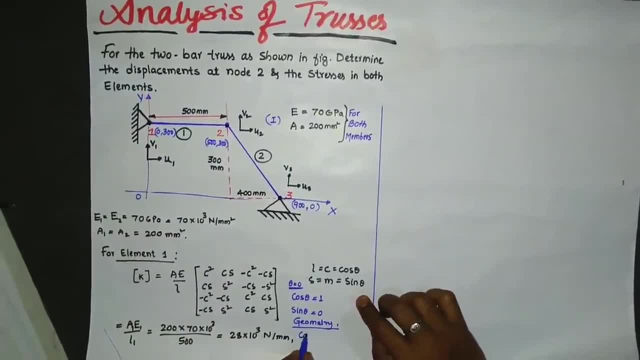 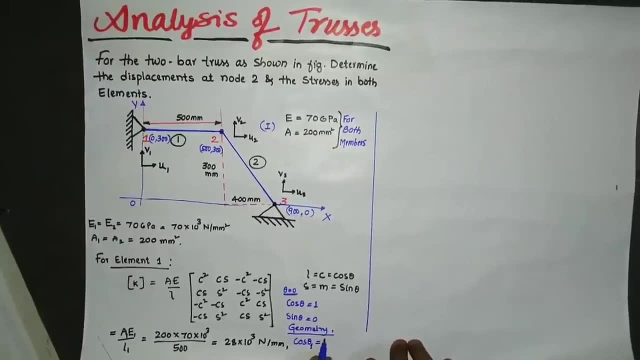 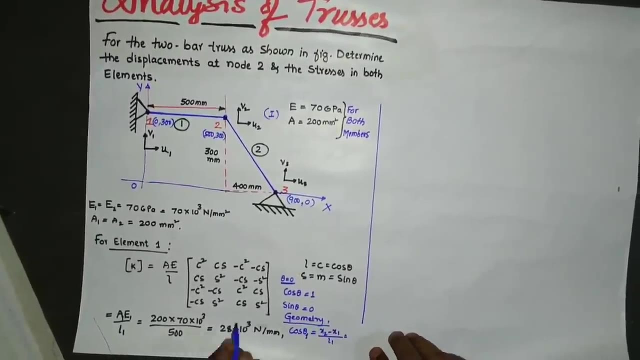 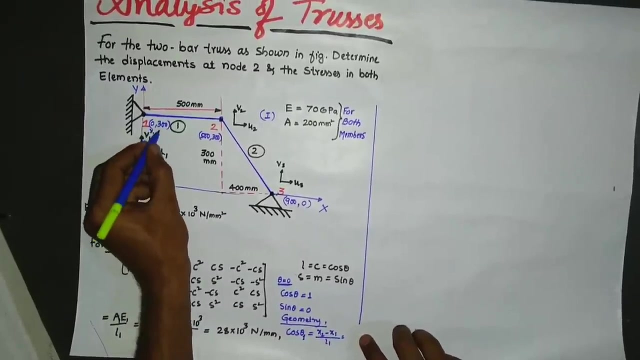 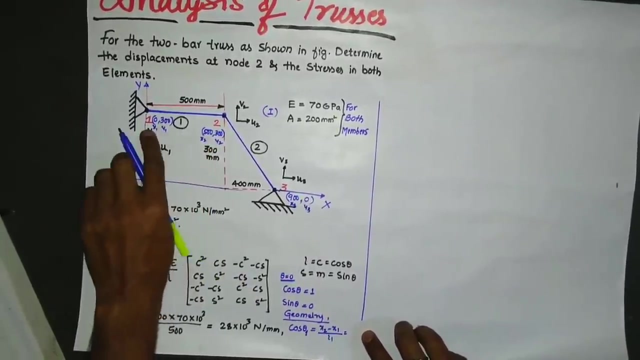 at the element one. so if you want to calculate cos theta one, so theta one is nothing but for element one. so there the equation. it will be x2 minus x1 by l1. so x2 value is: this is x2 is 500, so it is x1, y1, x2, y2, x3, y3, so larger minus the smaller one, x2 minus x1 means 500. 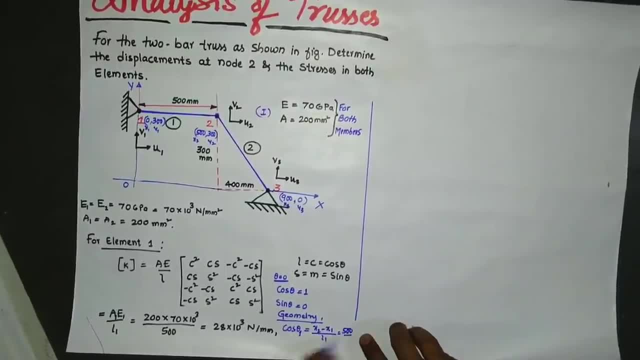 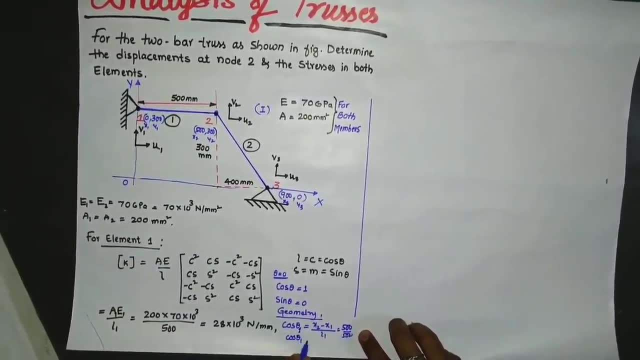 minus 0, so it will be 500 divided by the length of the element one, that is, l1 is 500. so we got cos theta 1 is equal to 1, same. so we have the same thing here. so we have the same thing here. 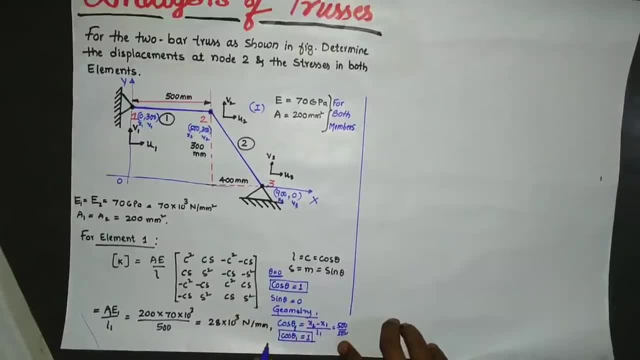 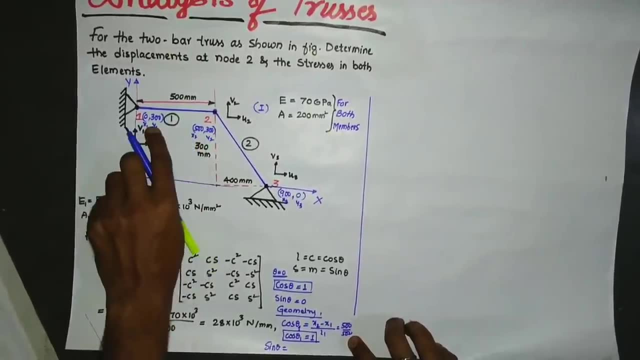 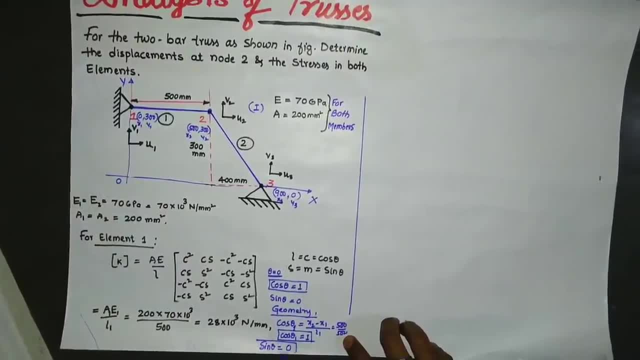 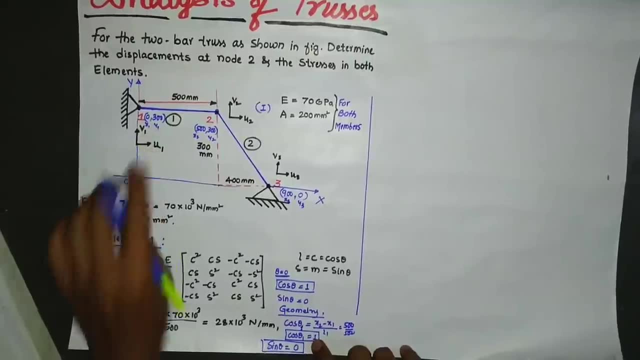 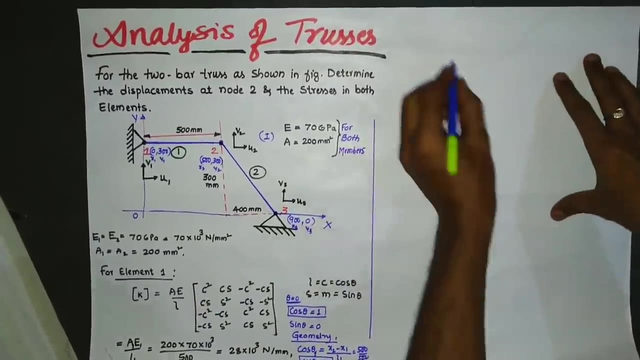 becomes 0, so sin theta is nothing but 0. so this is the second method. using that also you can calculate the cos theta and sin theta. so after that we will substitute in the k1 value. so with k1 is nothing but stiffness, matrix 1.. 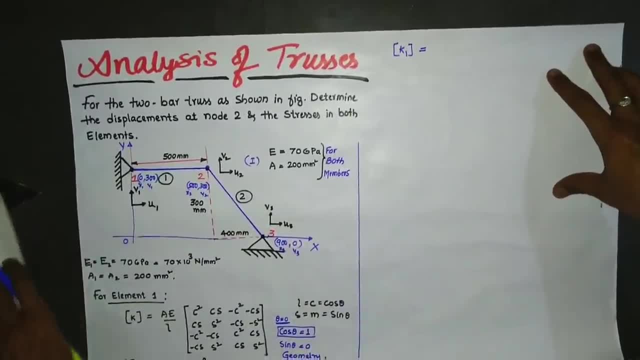 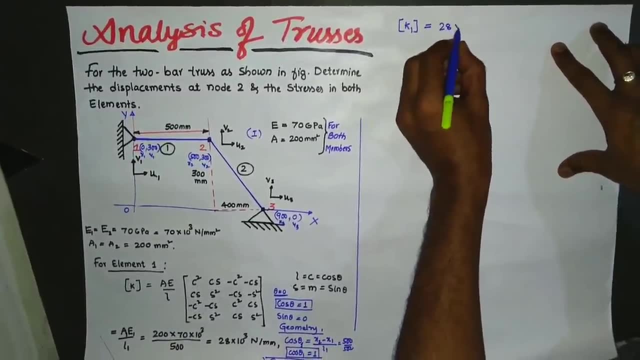 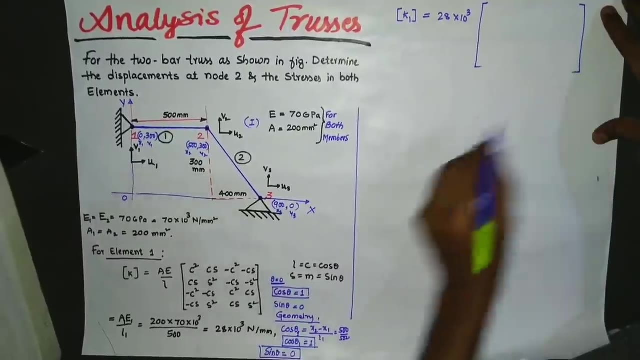 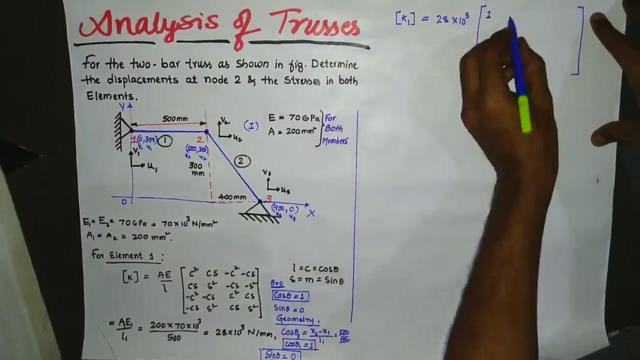 element 1.. so a by l is 28 into 10 to the power of 3.. again in the matrix, next c square. c value is 1. and one square is nothing but 1.. this is 1 into 0.. 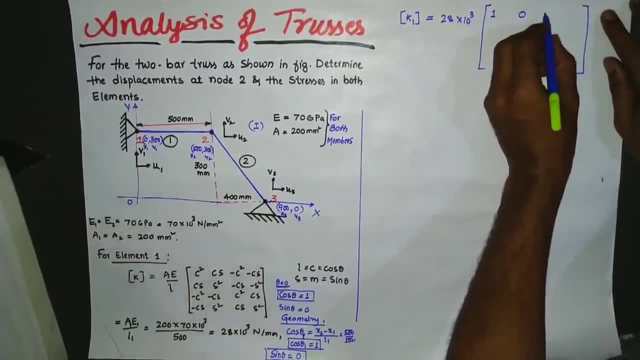 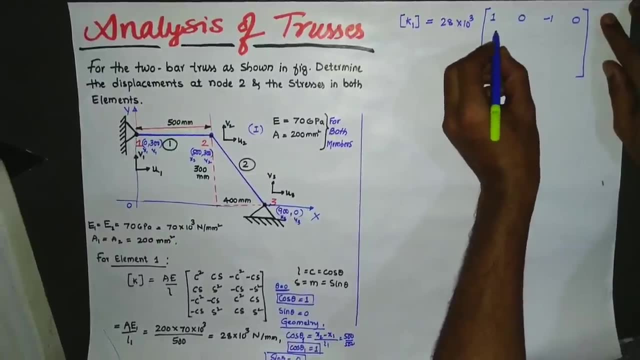 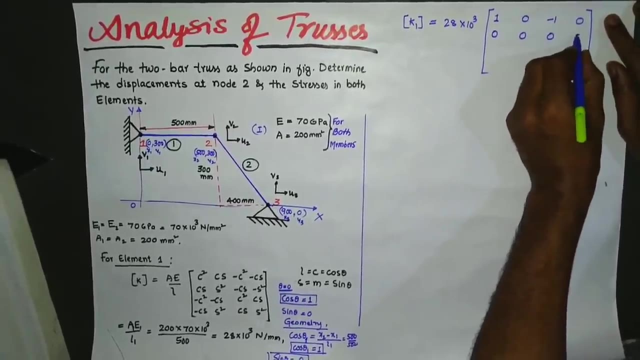 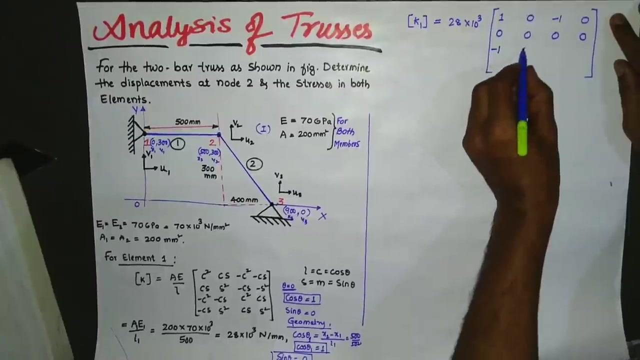 so it become zero. next minus c square. so it is again minus one. next c s is zero. similarly, we will calculate for c s again: zero s square, zero, c s. zero minus s square, also zero. similarly, third row: minus one c square minus c s is 0, c square is 1, c s is 0. so again c s 0 s. 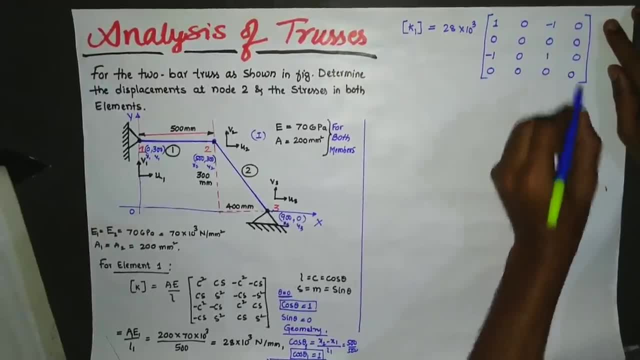 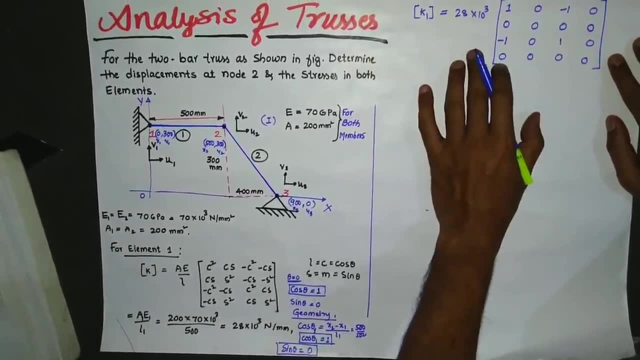 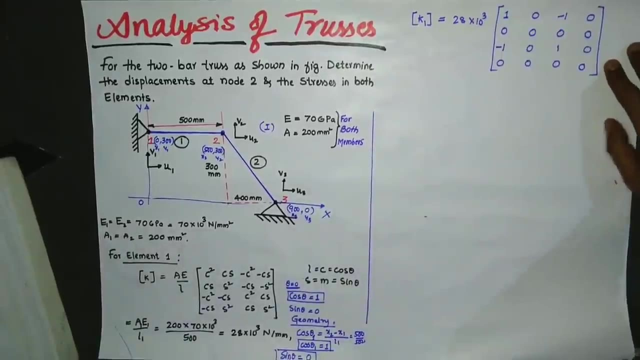 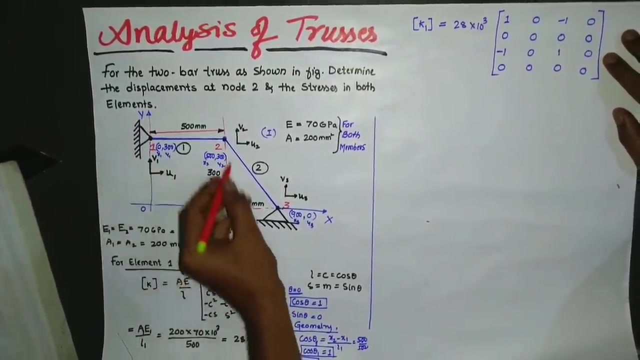 square, 0, c, s, 0, s square, it become zero. ok, so next for the element 1. this is the formation of stiffness matrix. so now you need to substitute the displacement for this matrix, so suppose at element 1.. so what are the displacement here? so it is u1, v1, u2, v2. so here it will be u1, v1, u2, v2. 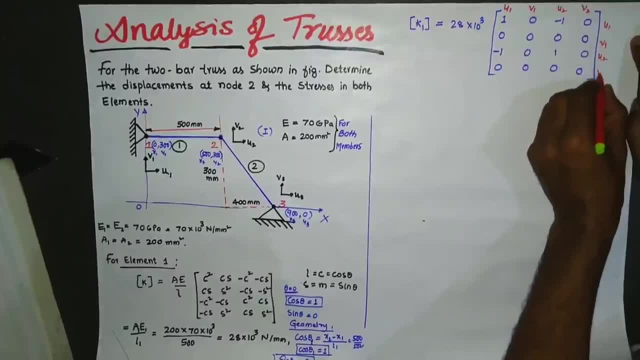 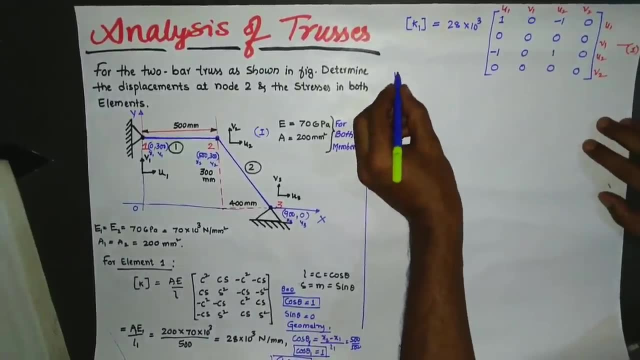 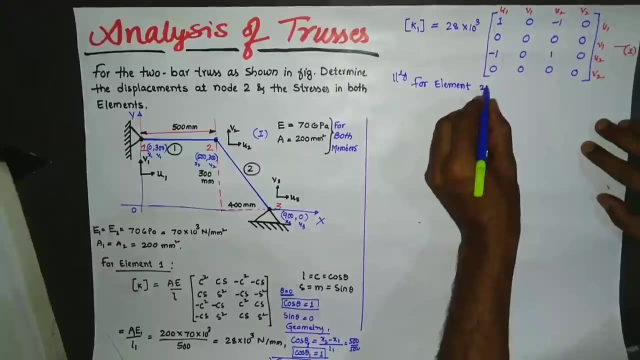 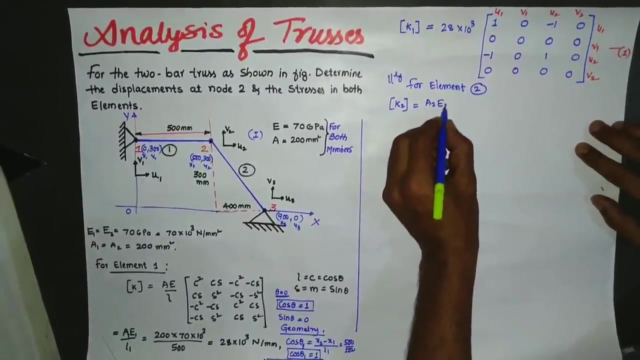 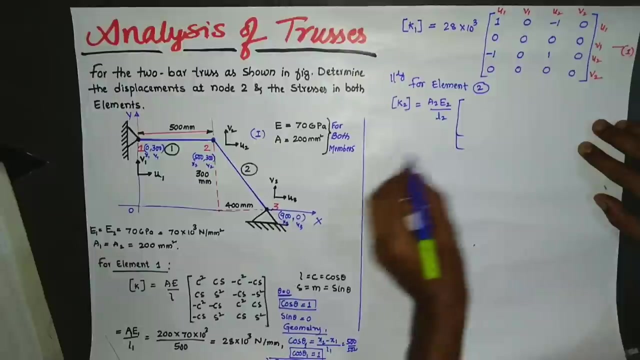 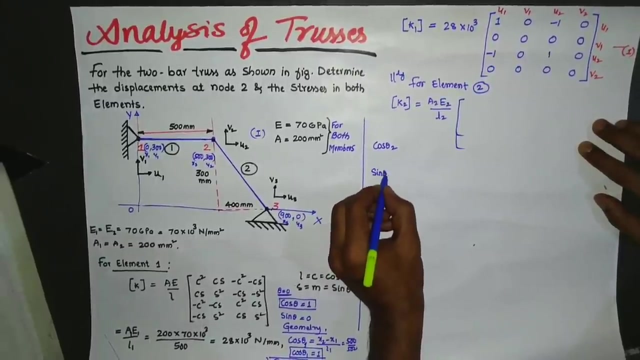 u1, v1, u2, v2. so let us say this is equation 1. similarly we will calculate for element 2, that is k2. so k2 is equal to again a2, e2 by l2. so same equation: it is c square cs. so now, before that you calculate what is cos theta 2 and sine theta 2. 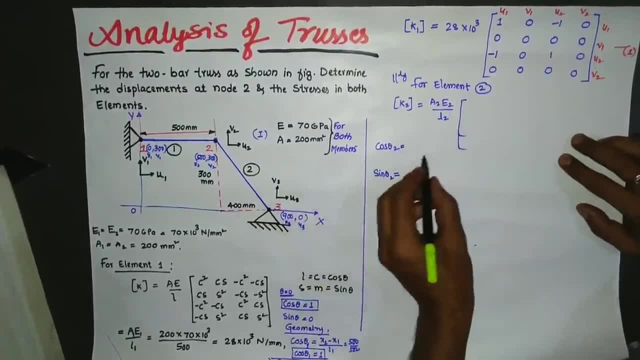 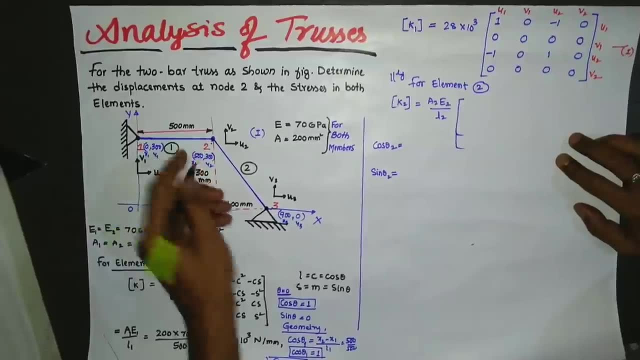 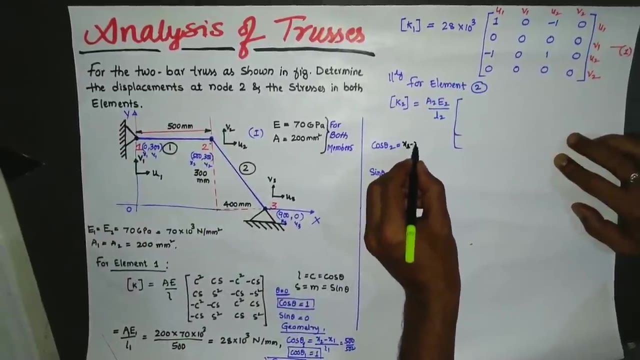 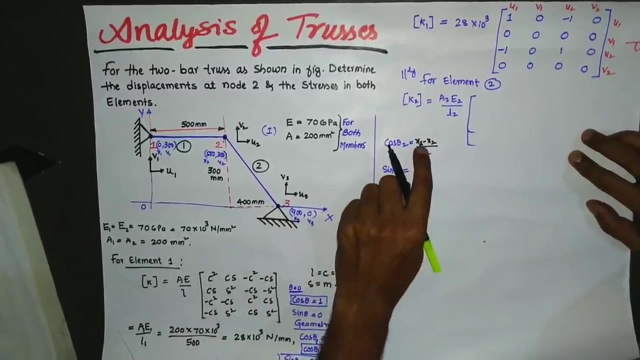 after this we will substitute the value within the matrix, so cos theta 2. so theta 2 is nothing but x3 minus x2. okay, so the connectivity it is from 3 to 2, so it will be x3 minus x2 divided by l2. so x3 value is 900 minus 500, so it will be 400. 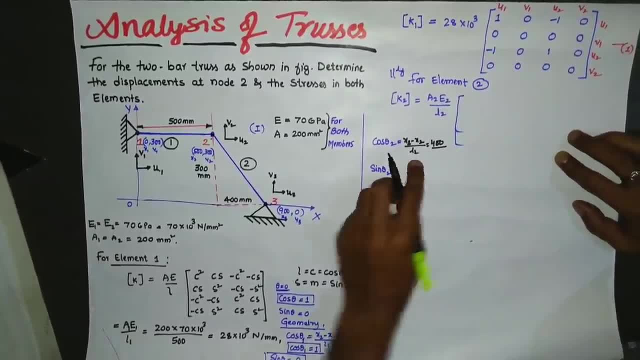 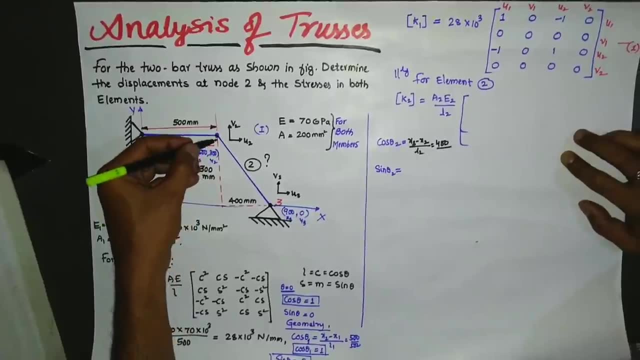 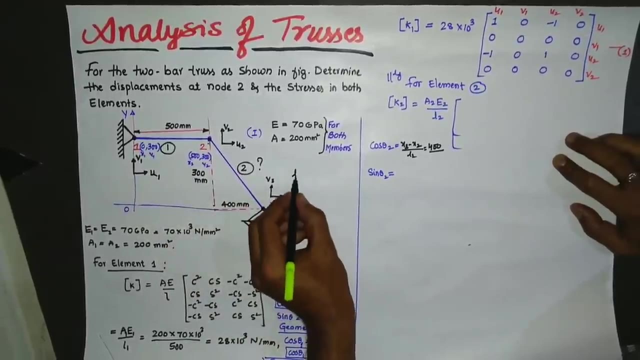 divided by the length for the element 2. so this is the length. so this length is not mentioned in the question, it is an unknown value. so but we have the opposite and the adjacent, so from the Pythagoras we can calculate the L2. so 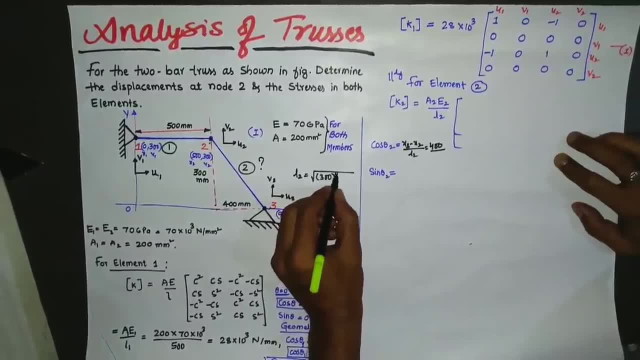 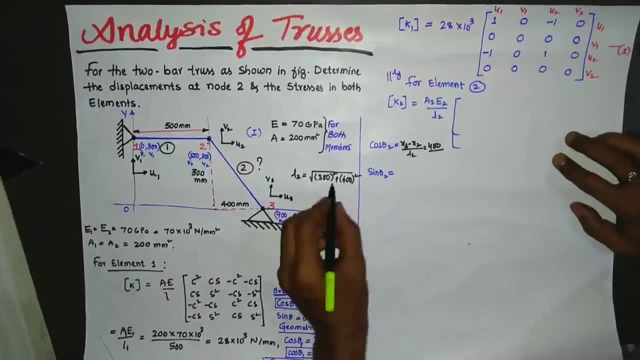 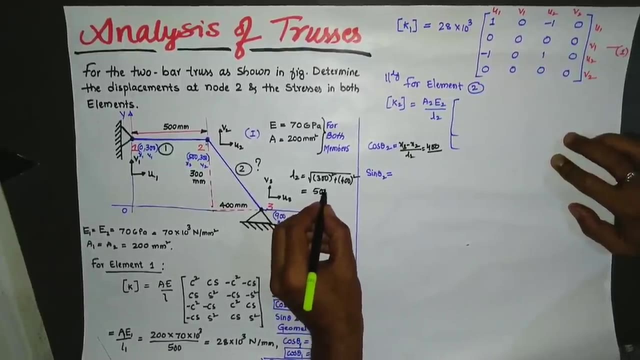 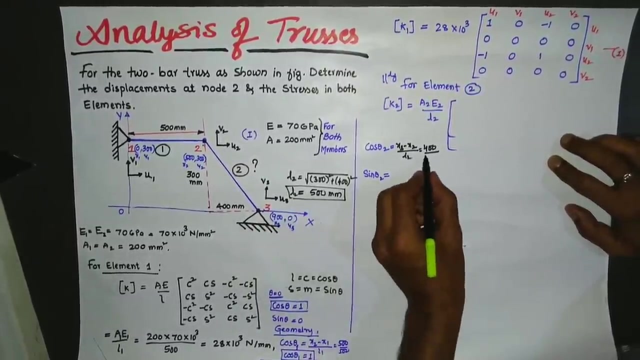 where L2 is equal to 300 square plus 400 square, so nine hundred nine thousand plus 16,000, so 25,000. so 25,000 is equal to square root of 25, so 500 millimeter is the length for element 2, so now 500. so 400 divided by 500 is: 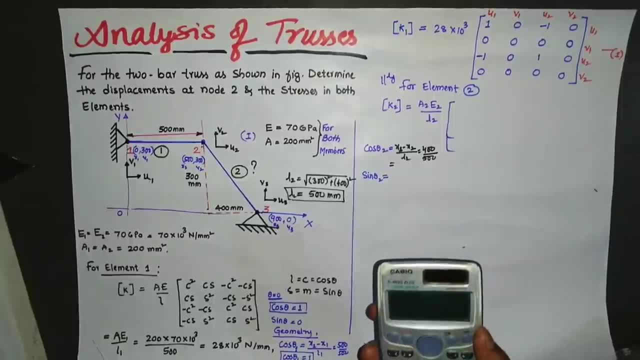 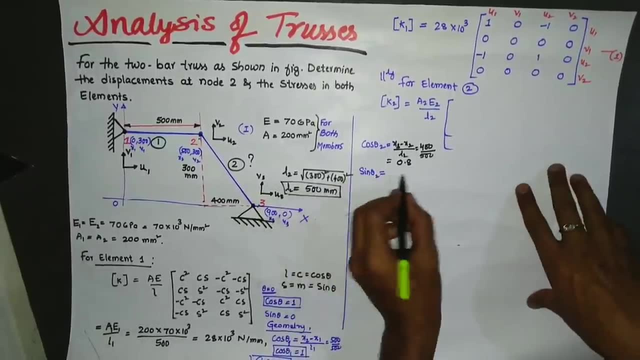 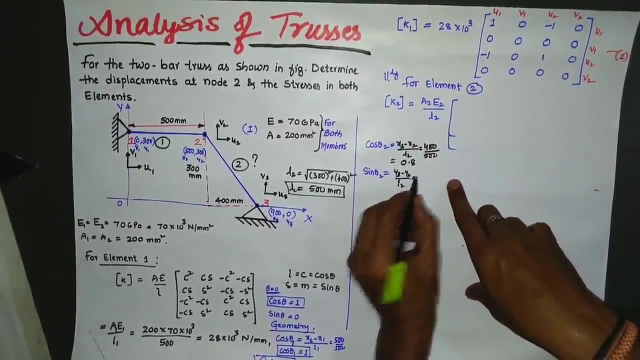 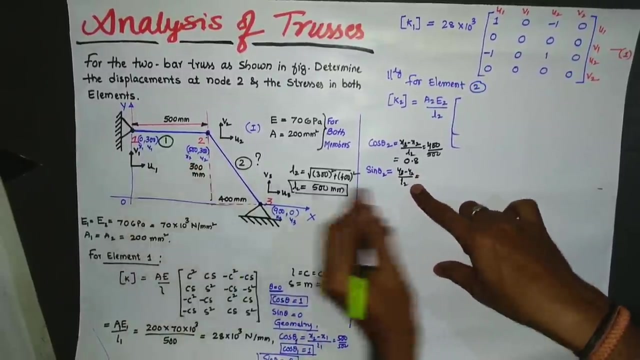 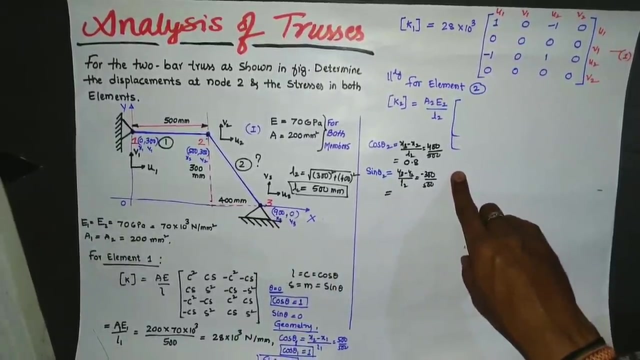 equal to 0.8 is cos theta 2. similarly, for sine theta 2 it is y 3 minus y 2 divided by L 2. so y 3 value is 0 minus 300. so minus 300 divided by 500 is equal to minus 0.6. 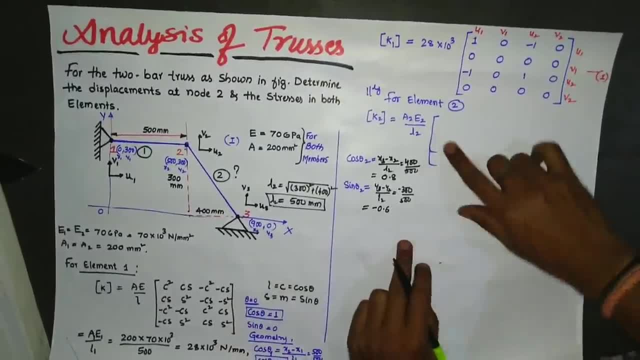 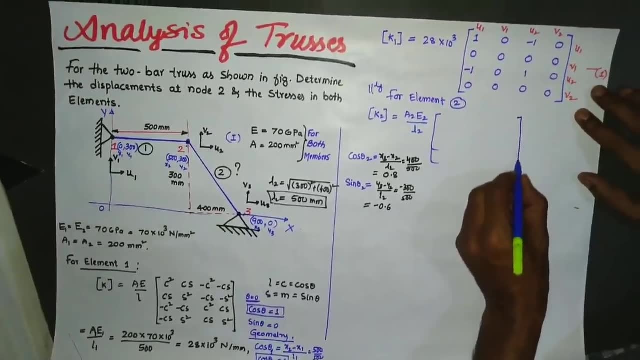 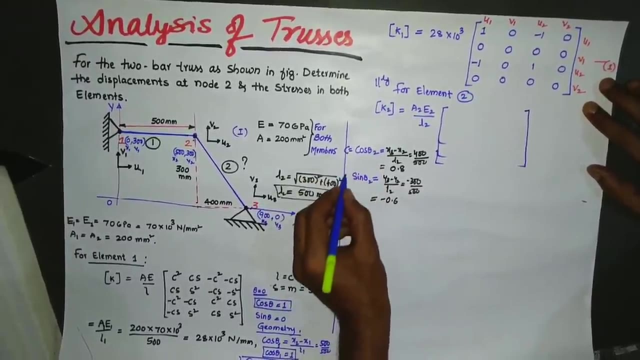 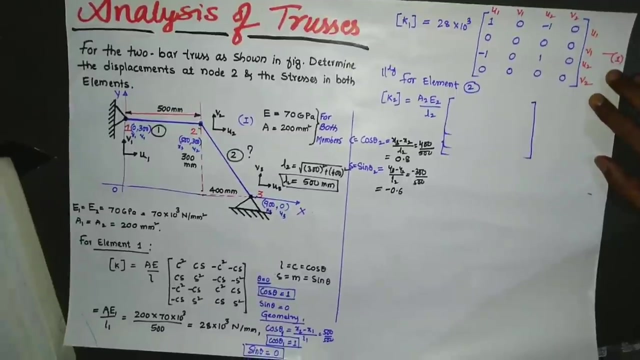 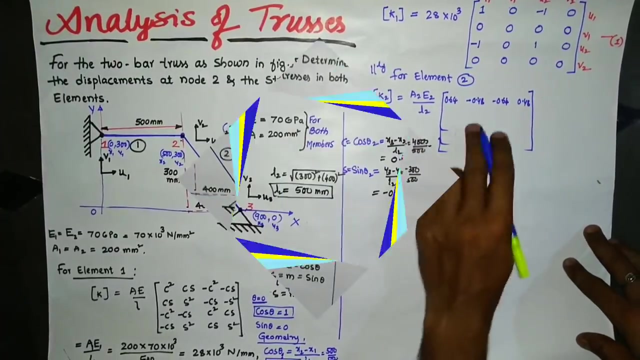 is sine theta 2, so we will take the. this value will make the in the matrix okay. so c square c, it is nothing but c, and this is s, so c square 0.8. so 0.8 is nothing but 0.64 is the value for c square. 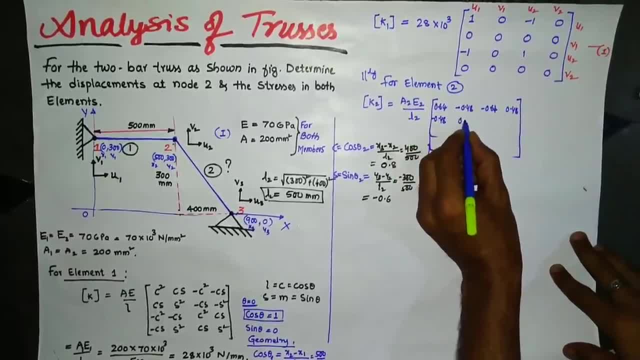 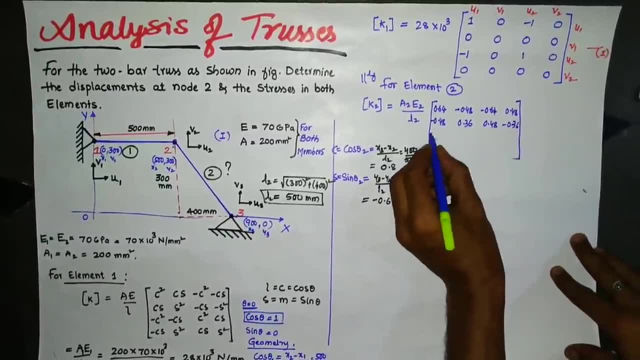 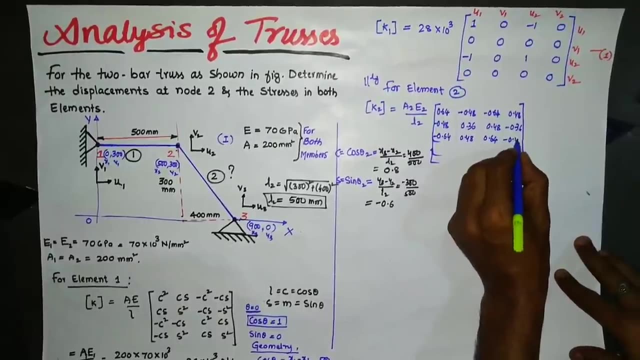 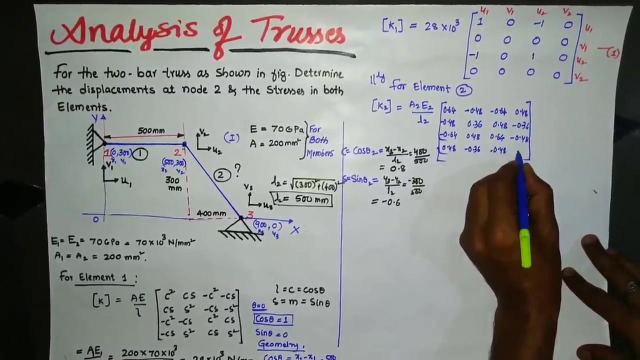 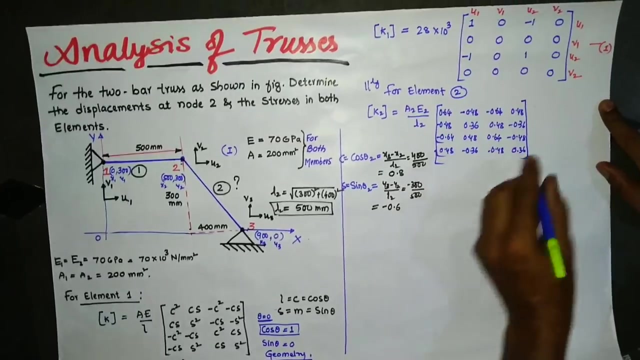 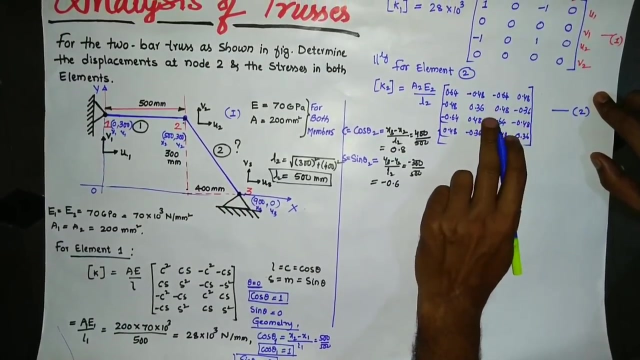 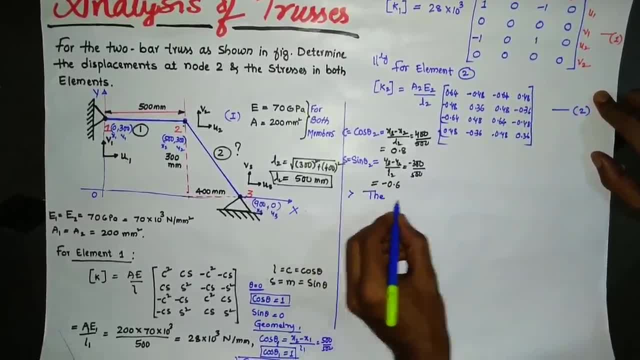 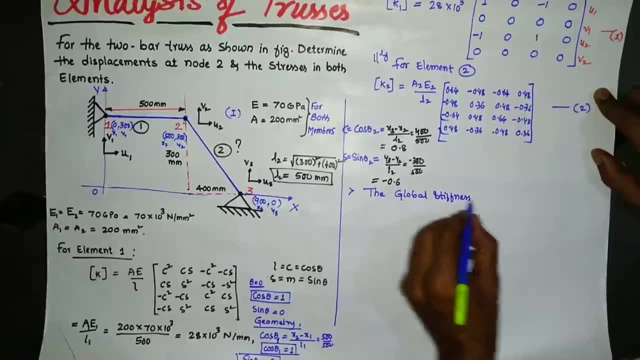 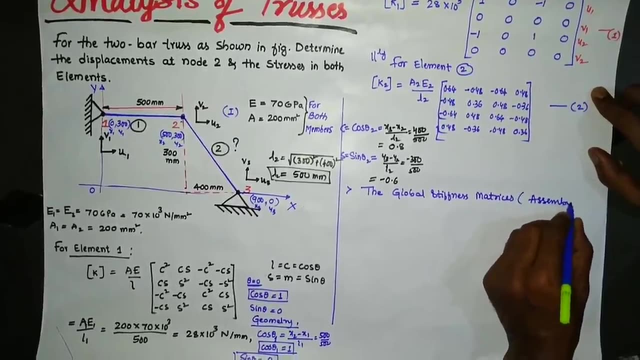 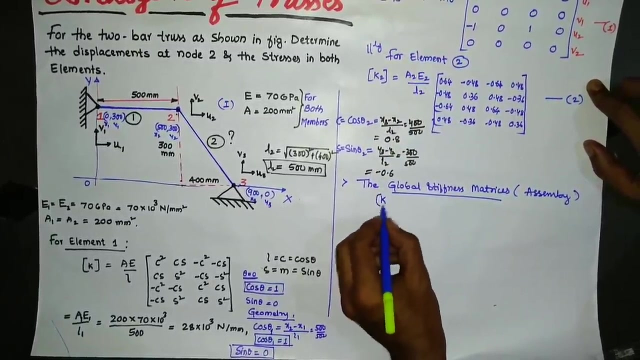 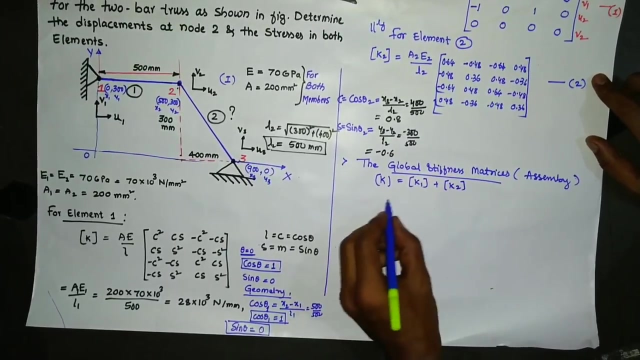 then the next step is to calculate the global stiffness matrix. global stiffness matrix, so the global stiffness matrix, it is nothing but assemble, assembly of all the stiffness matrix. so we have two elements of this, that is, k1 plus k2. so we have to add the global stiffness matrix. and one more thing we have not calculated: 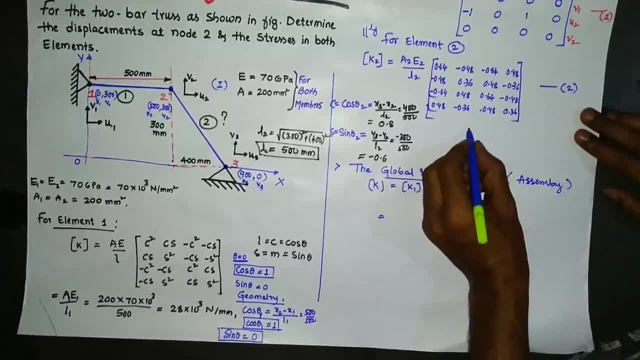 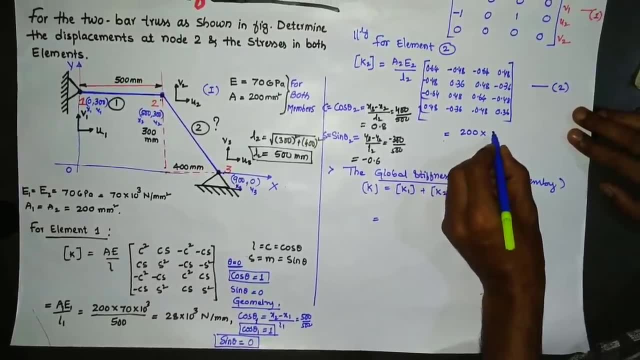 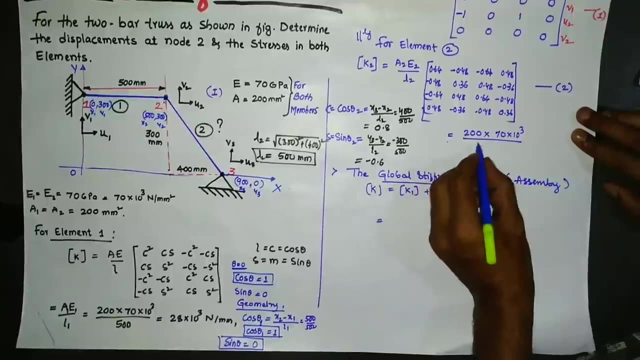 here a2, e2 by l2, so that also we will calculate. now it's equal to a2. value is again same, that is: e2 is also 70 x 10. power of 3 divided by the length for the element two, that is again 500. 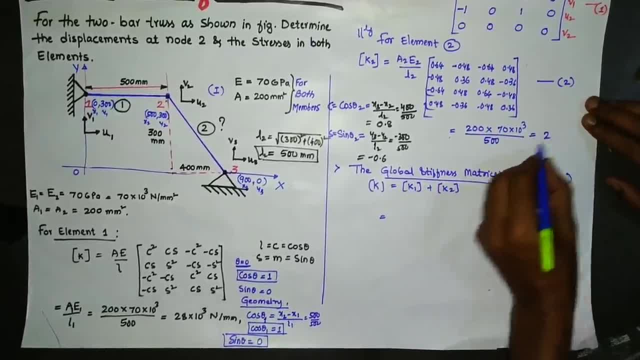 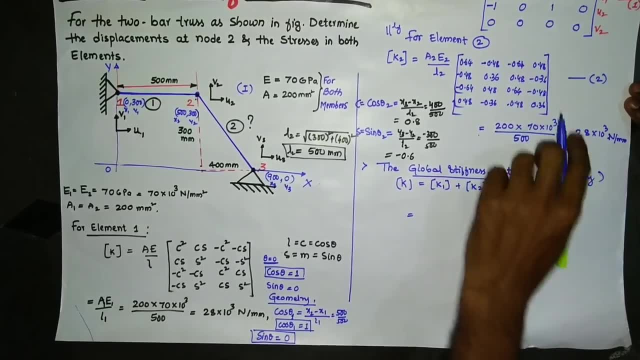 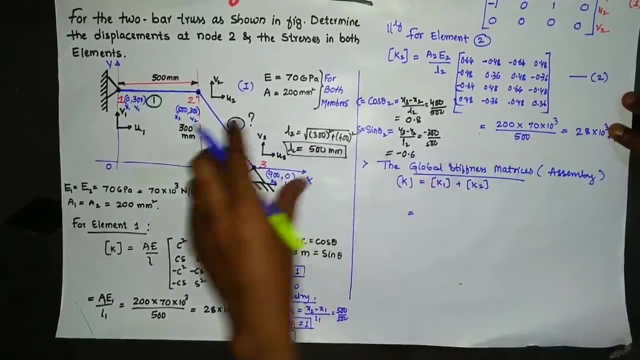 so this is equal to: again we have the same value, that is, 28 x 10. power of 3 Newton per millimeter: see for element one is also 28 into 10. power of 3 Newton per millimeter: see for element 1 is also 28 and for element 2 also 28, because we got the same value. it is: 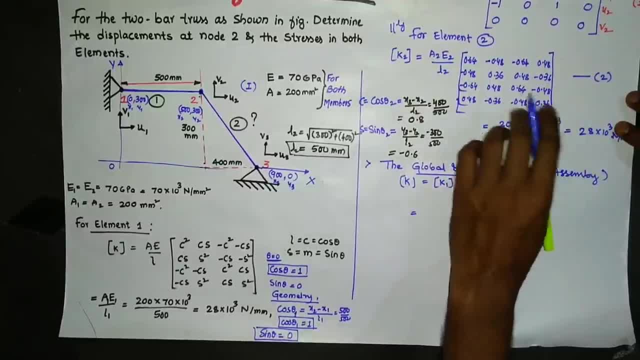 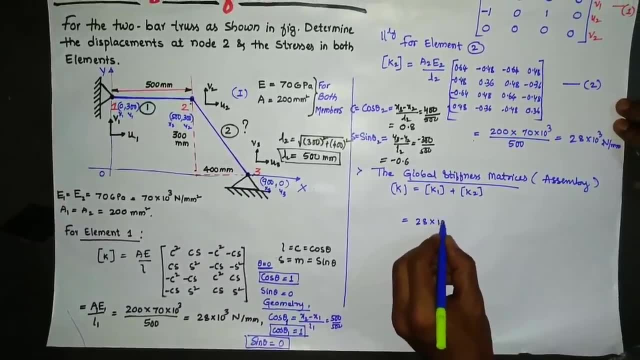 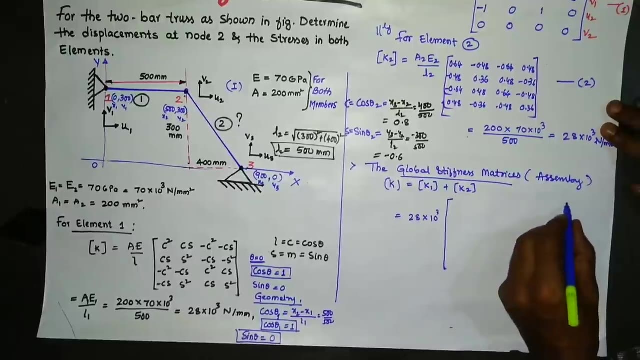 not that it not mean that it should be same. okay, so we got the same value. so it is easy to take the common term. so 1028 into 10, power of 3, we will take as a common for both the elements. now to assemble these two matrix, we have to write all the displacement first. 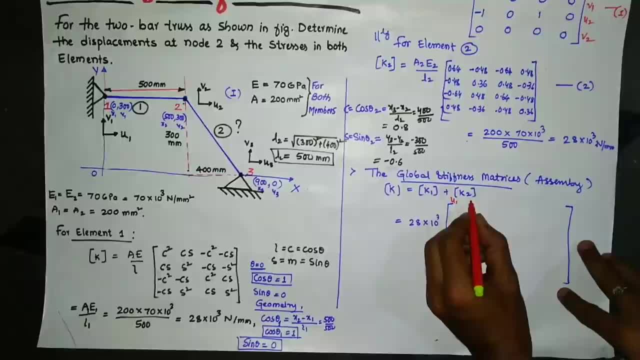 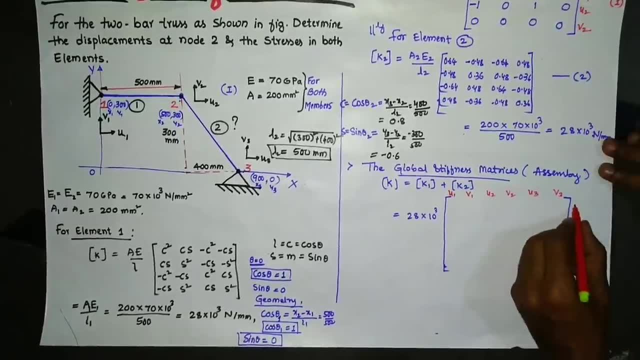 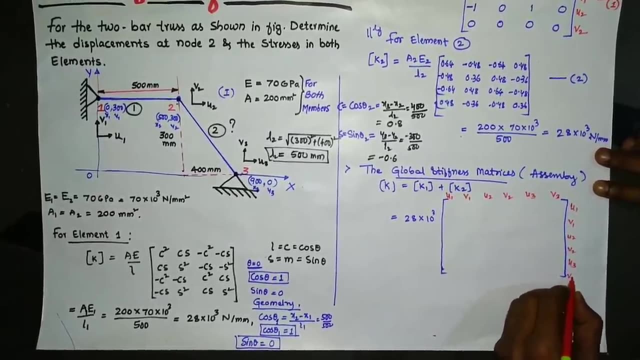 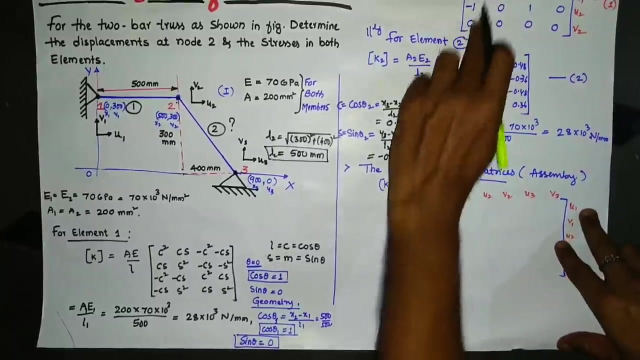 so let us write the displacement outside the matrix: u1b1, u2v2 a, u3b3. similarly in the row also u1b1, u2v2 a, u3v3. okay, So after that. so after that will add the value from the element 1 and element 2. suppose you have u1 in the row and 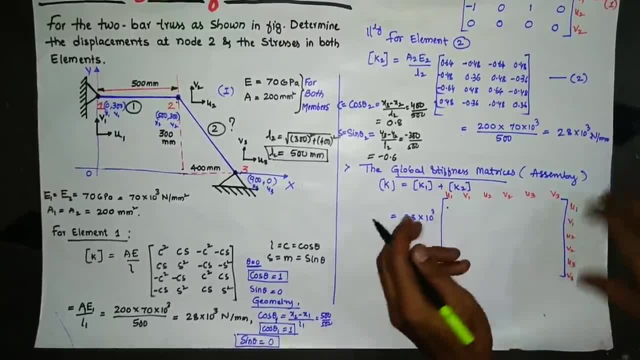 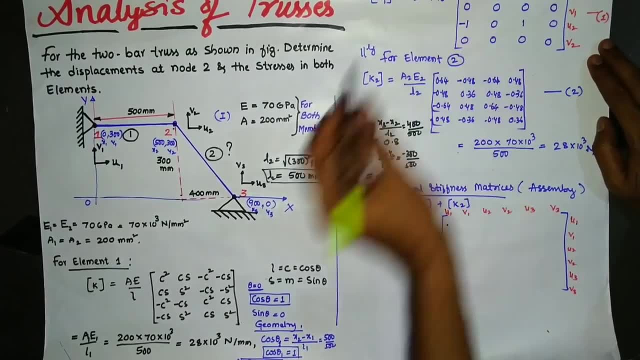 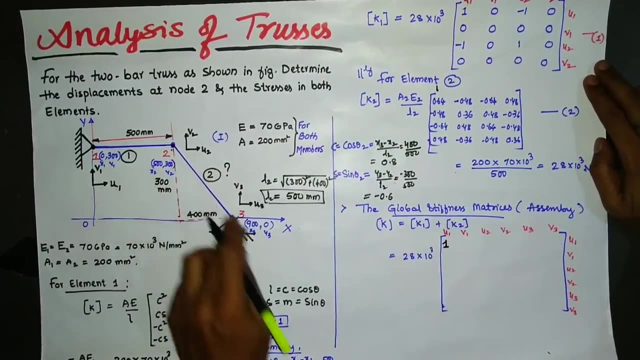 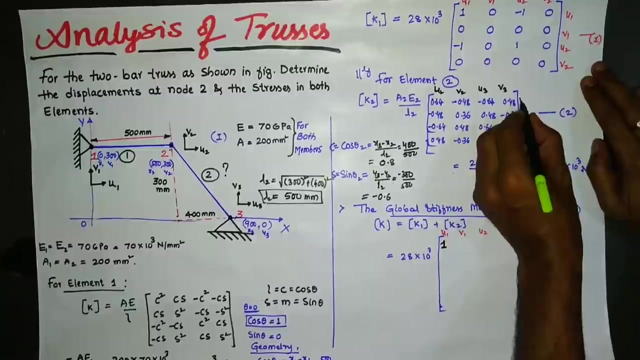 in the column again one more: u1. so what value we can get it here? so you have to see the element 1 here: u1, u1. that value is 1, so it should be 1 here. so at the element 2 there is. so here again for element 2, it is u2, v2, u3, v3. for element 2: u2, v2, u3, v3. so here there. 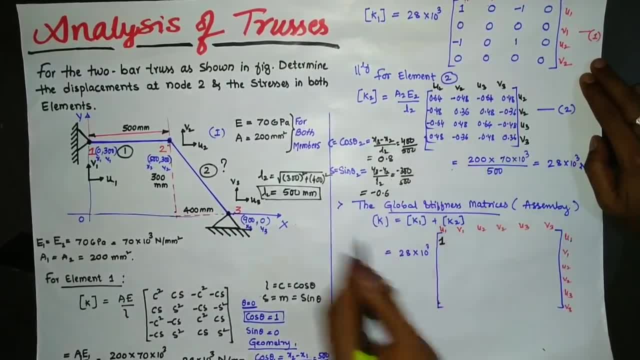 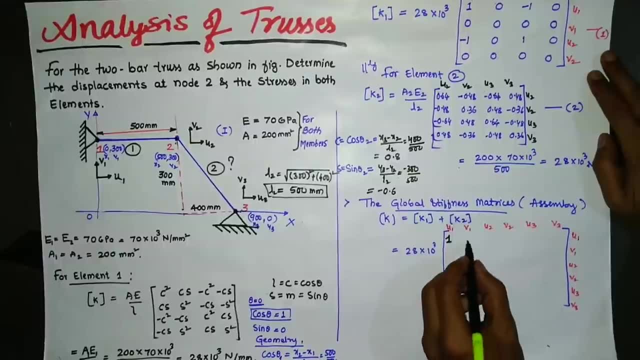 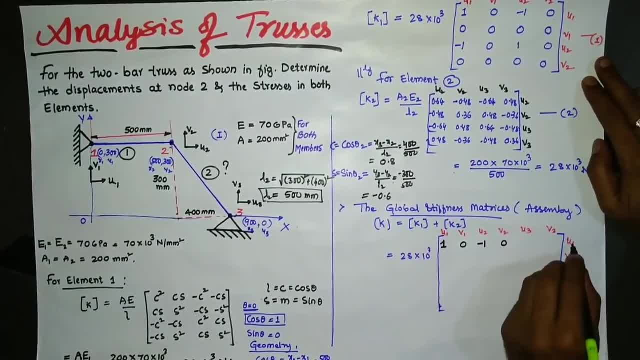 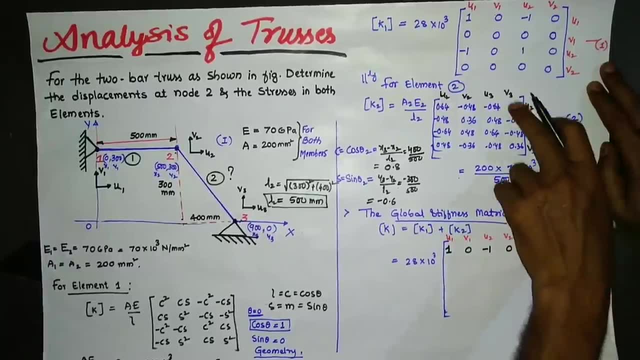 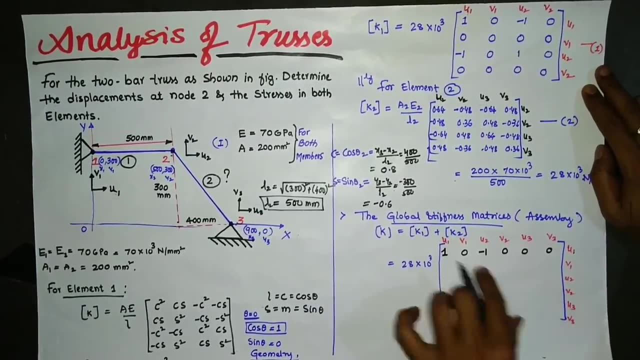 u1- u2 is minus 1. u1- v2 is 0. so u1- u3- so near no relation for the u1 and u3 at 1 and here also at 2, also no relation, so it will be 0: 0, like that you have to calculate for all the matrix. okay, so due to the 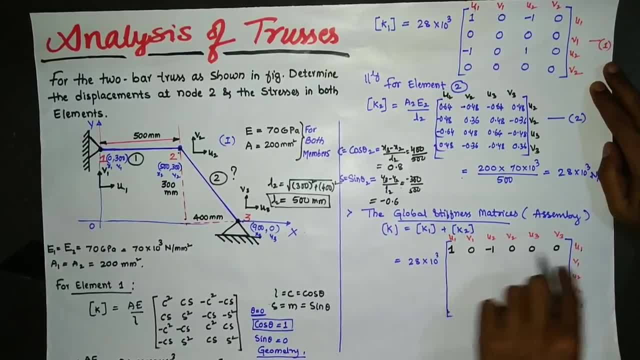 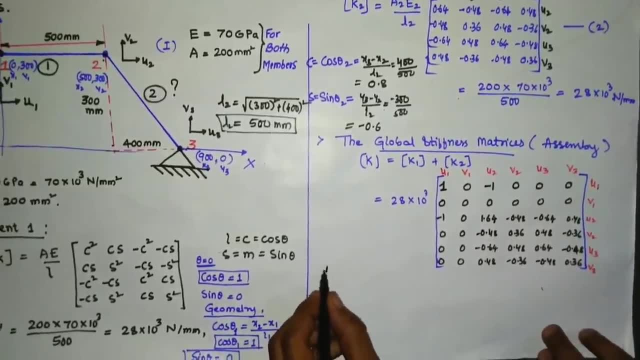 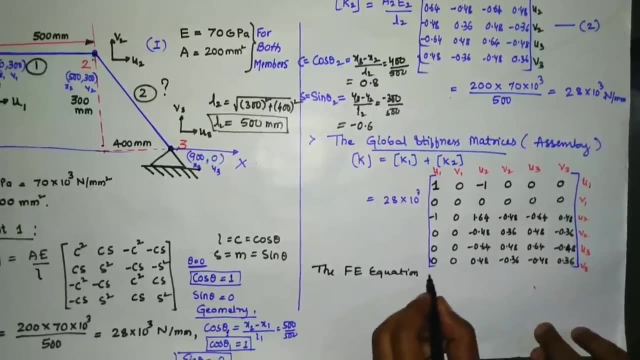 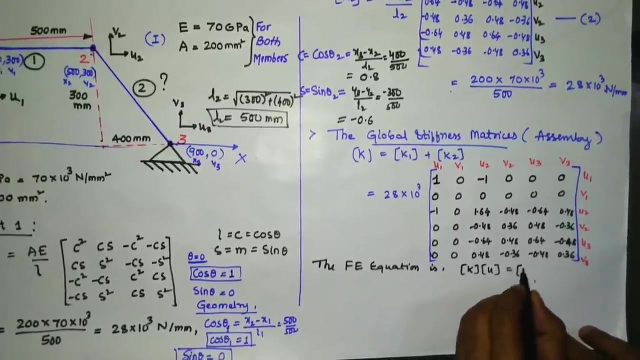 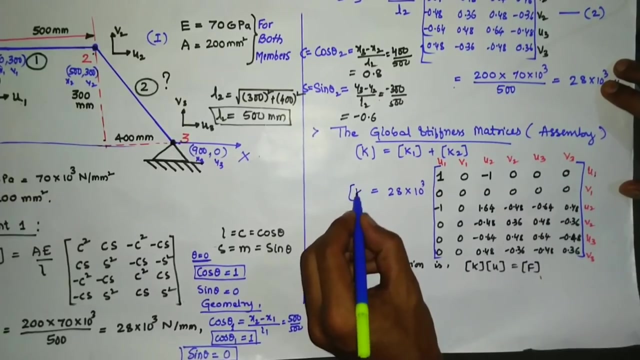 lack of timing, i am just substituting the value so you can check this answers. so after that, the finite element, equation, matrix equation is that is k? u is equal to f, so this formation you have to make. so k? u we have already calculated. so this is nothing but k value for now, the displacement matrix. 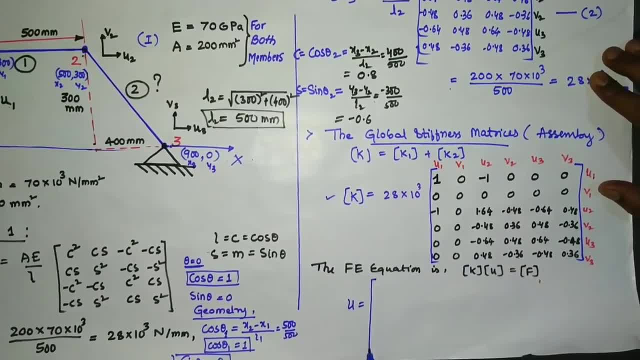 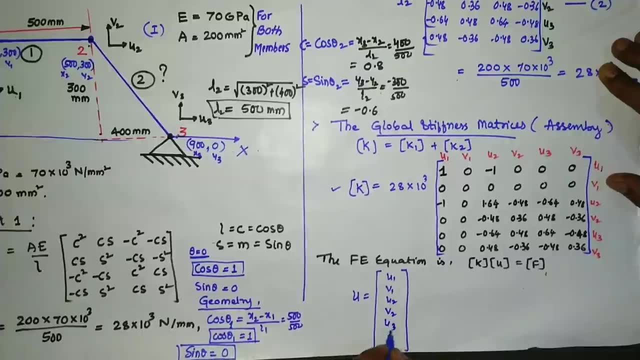 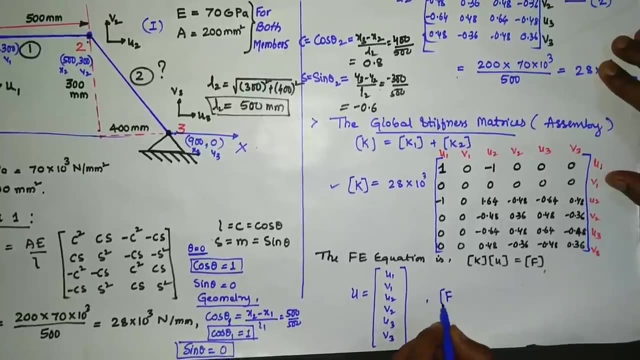 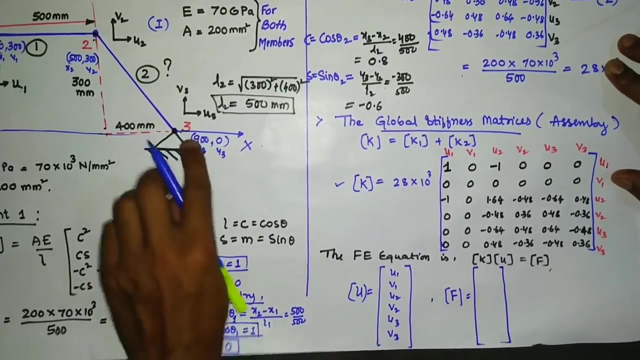 it is u, so you have to write all the displacements, that is, u1, v1, u2, v2, u3, v3 are the total number of displacement. according to the problem now, the force vector, so f, is equal to, so in the truss element. so in the truss element again, there will be two types. 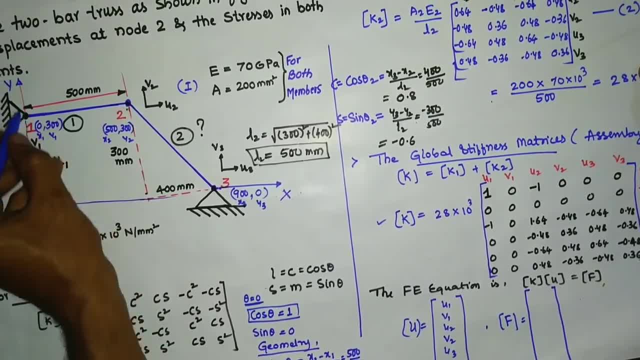 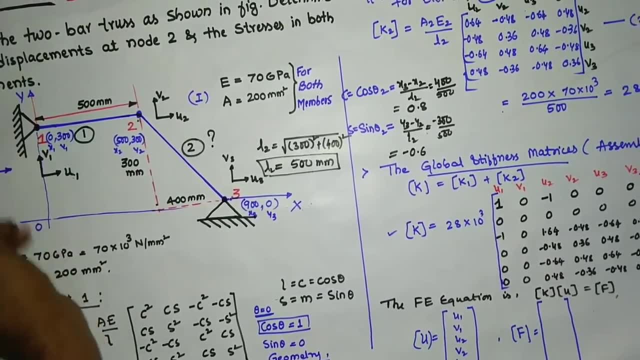 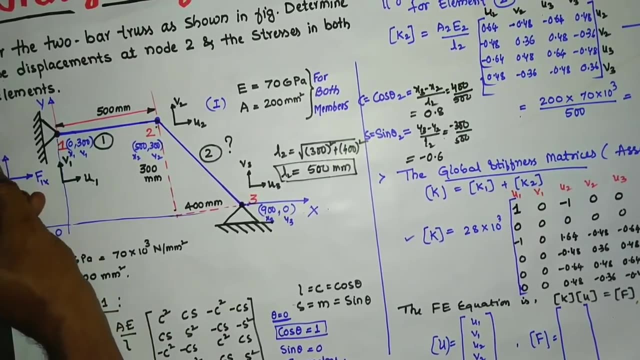 of no loads at each nodes, suppose at the node 1, you think it is at the node 2, so you think it will be node 1. we will have one, it will be horizontal force, another and vertical force. for horizontal, we will represent f1 x for the horizontal, at vertical f1 y. similarly at 2, also f2 x. 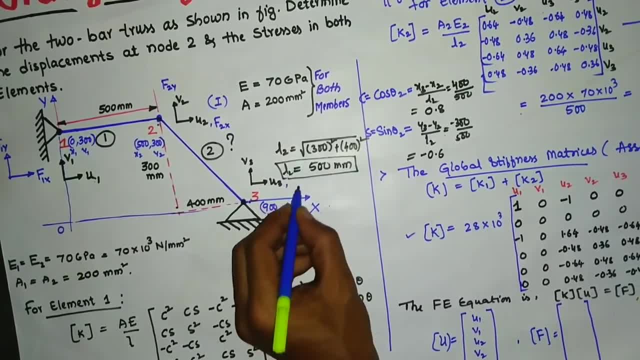 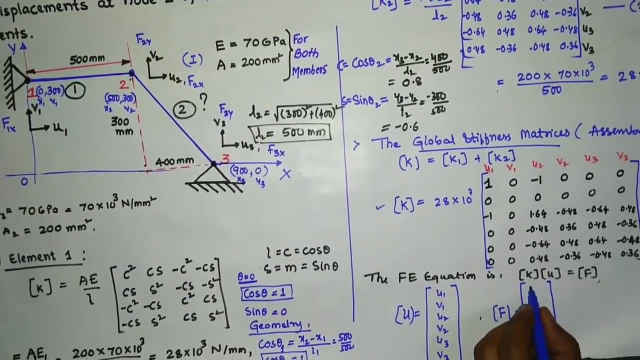 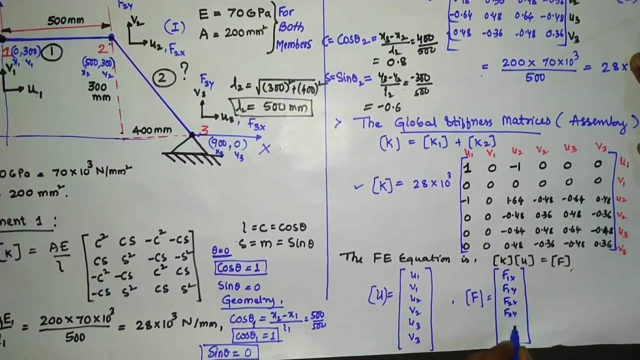 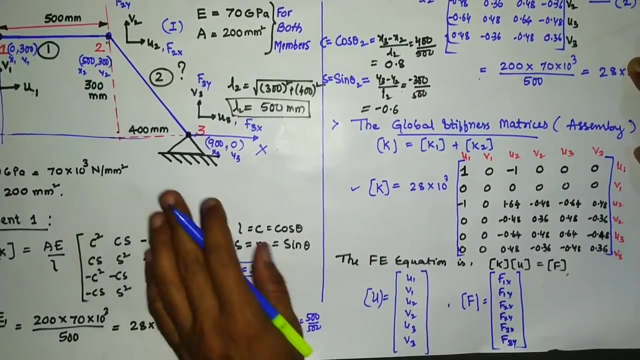 f2 y, at 3, f3 x, f3 y are the forces, same forces. you write down here: f1 x, f1 y, f2 x, f2 y, f3 x, f3 y. so these are the forces. now are the boundary conditions. okay, so boundary condition. 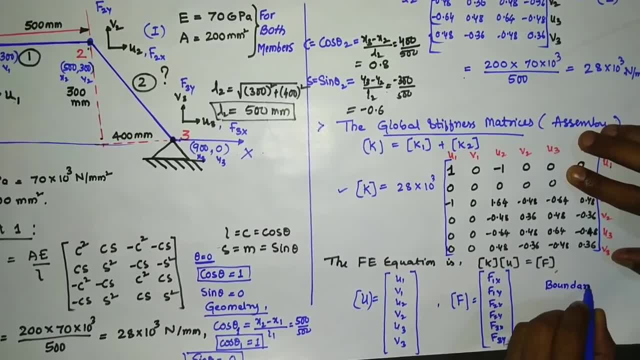 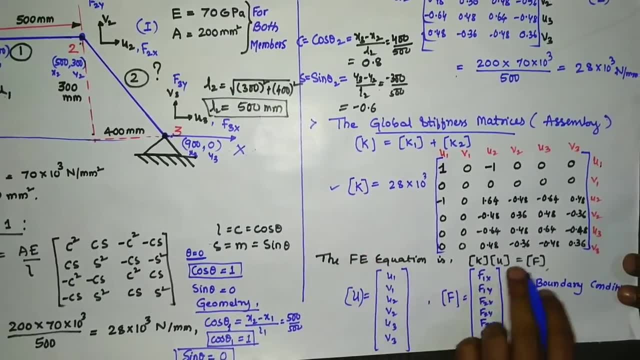 for this problem. okay, so boundary condition for this problem. okay, so, boundary condition for this problem. so what are the boundary condition? so first thing is that you have to make in. so what are the boundary condition? so first thing is that you have to make in. so what are the boundary condition? so first thing is that you have to make in this formation. 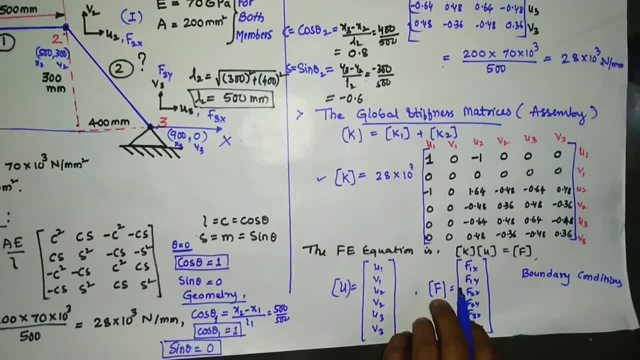 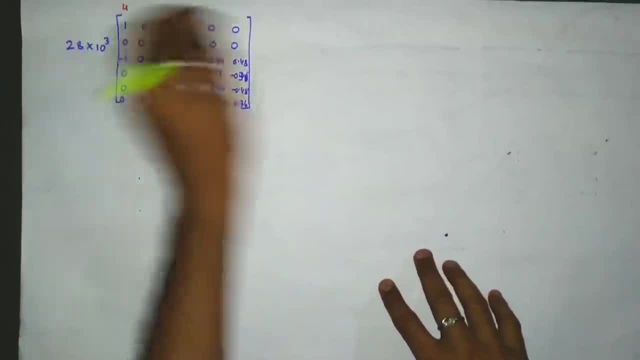 this formation, this formation. later we will apply the boundary conditions. so this is the stiffness matrix which i so. this is the stiffness matrix which i so. this is the stiffness matrix which i have written just now, have written just now, have written just now. so this is the displacement is u1. 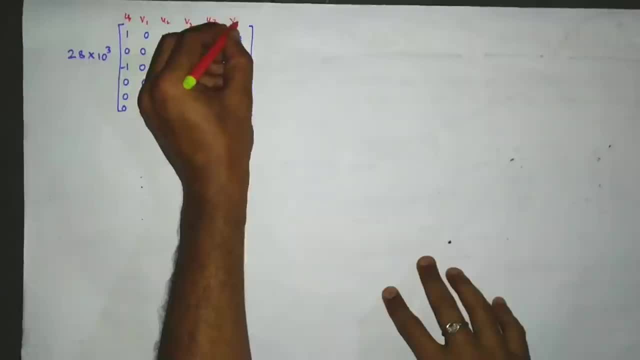 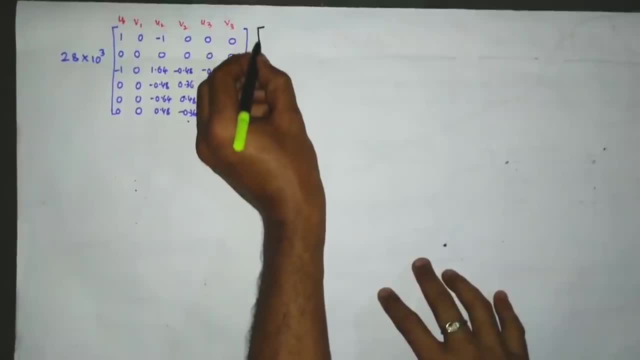 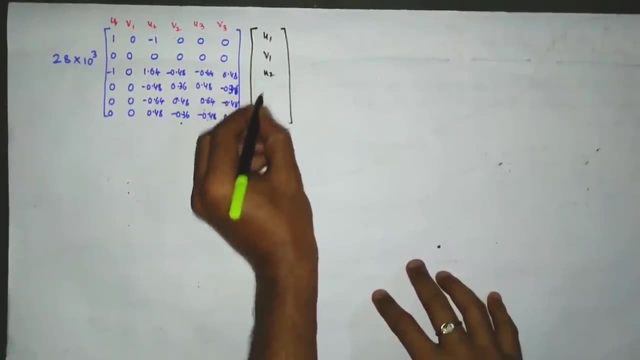 v1, u2, v2, u3, v3. similarly, you will write the. similarly, you will write the. similarly, you will write the displacement vector. that is displacement vector. that is displacement vector. that is u1, v1, u2, v2, u1, v1, u2, v2, u3, v3. 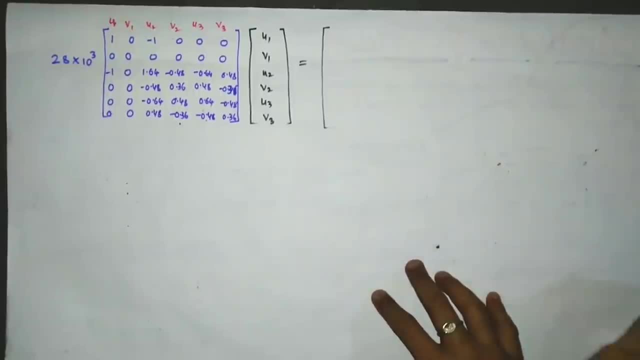 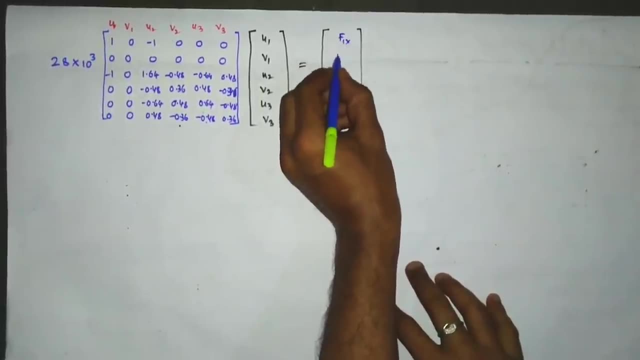 u1, v1, u2, v2, u3, v3, u1, v1, u2, v2, u3, v3. is equal to the force vector. is equal to the force vector. is equal to the force vector f1 x, f1, f1 x, f1 y. 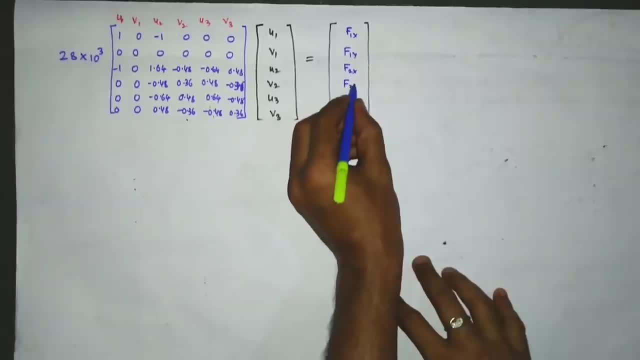 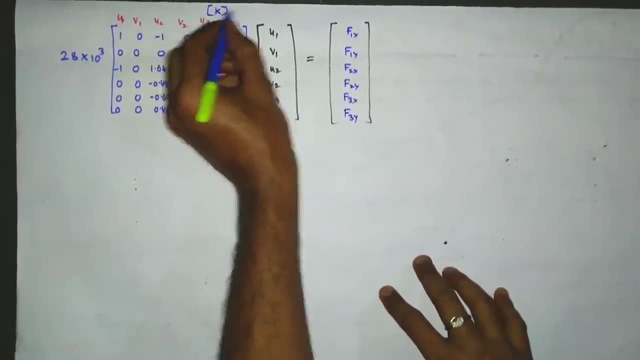 f1 x, f1 y, f1 x, f1 y, f2 x, f2 y, f3 x, f3 y. okay, so is as f2 x, f2 y, f3 x f3 y. okay, so is as f2 x, f3 x, f3 y. okay, so is as equal to K? u is equal to this formation we have. 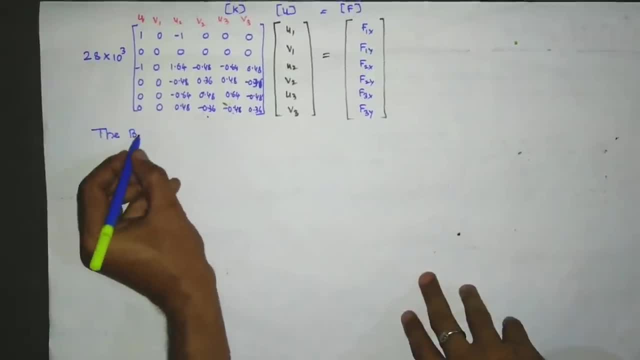 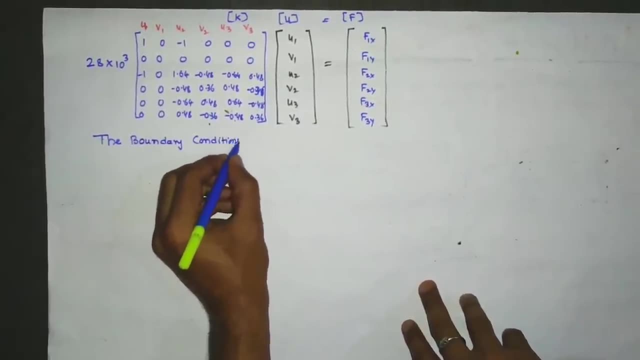 equal to K? u is equal to this formation we have. equal to K? u is equal to this formation. we have made it so now after that. so the made it so now after that. so the made it so now after that. so the border conditions are, border conditions are. 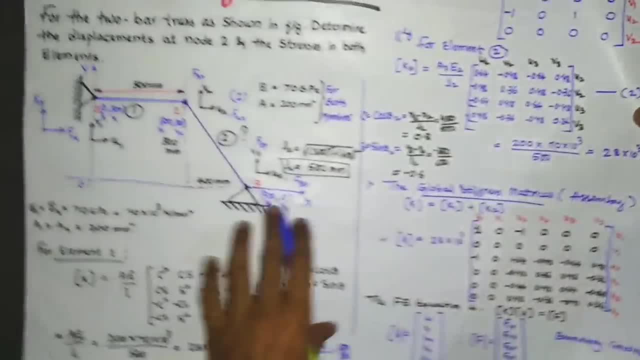 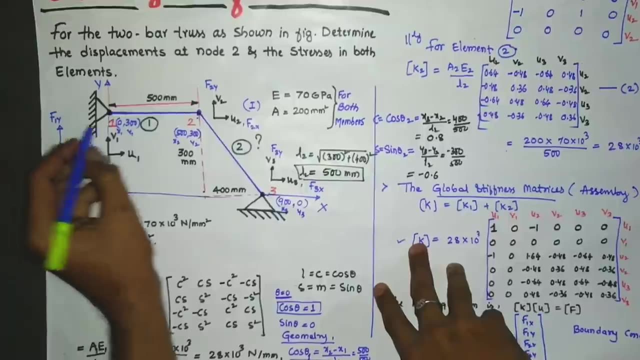 border conditions are. so from the geometry we will go for the. so from the geometry we will go for the. so from the geometry we will go for the geometry. so here at the node 1, there the geometry. so here at the node 1, there the geometry. so here at the node 1, there the x1 and v1 is will be 0 because at hinge. 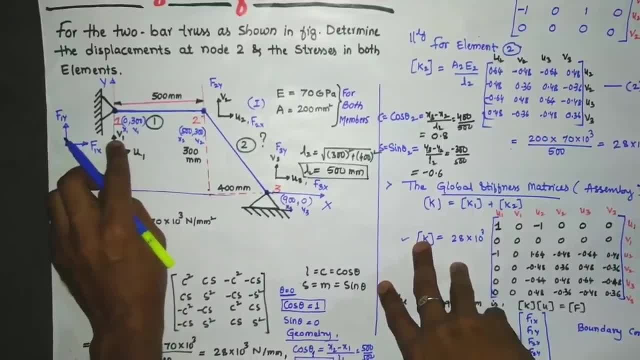 x1 and v1 is will be 0 because at hinge x1 and v1 is will be 0 because at hinge node. so there will be no horizontal node, so there will be no horizontal node, so there will be no horizontal displacement and also vertical if it is. 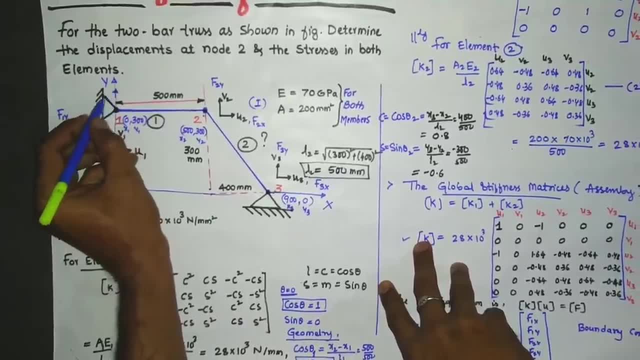 displacement and also vertical if it is displacement, and also vertical. if it is an roller support, then there will be an an roller support, then there will be an an roller support, then there will be an vertical displacement. if, in case of roller, vertical displacement. if, in case of roller, 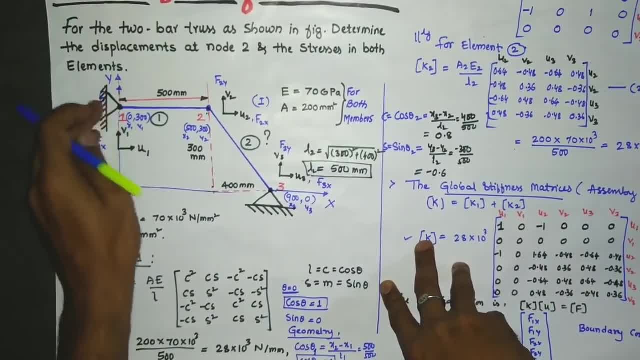 vertical displacement. if, in case of roller, okay, so roller means it can slides. okay, so roller means it can slides. okay, so roller means it can slides in the vertical, but it cannot slides in the in the vertical. but it cannot slides in the in the vertical, but it cannot slides in the horizontal. so that will be the 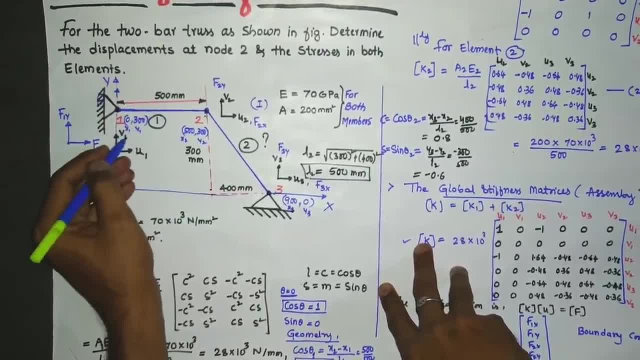 horizontal. so that will be the horizontal. so that will be the concept here. okay, so it means u1 v1 is 0. concept here. okay, so it means u1 v1 is 0 concept here. okay, so it means u1 v1 is 0. similarly at another node. 3 is also. 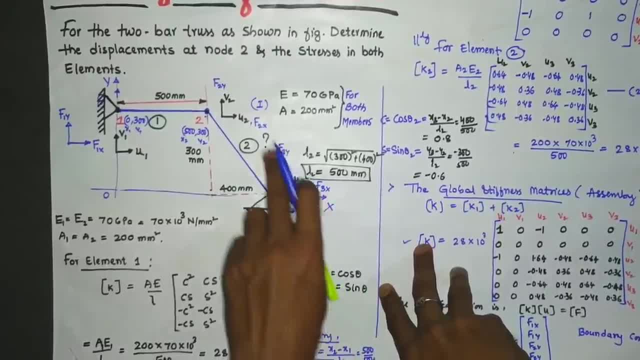 similarly at another. node 3 is also similarly at another. node 3 is also hinged support. so there also u3 v3 0 but hinged support. so there also u3 v3 0 but hinged support. so there also u3 v3 0, but yet node 2 it is free. so u3 and sorry. 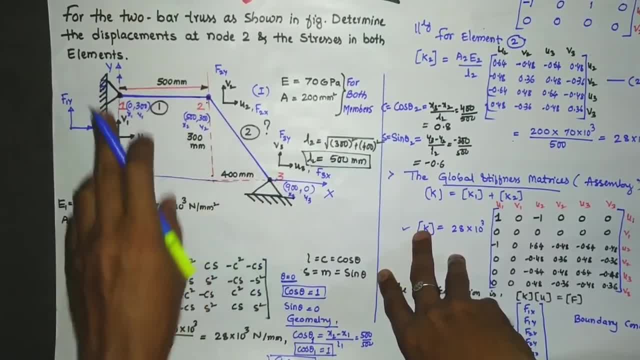 yet node 2 it is free. so u3 and sorry. yet node 2 it is free. so u3 and sorry. u2 v2 will have the values and also the u2 v2 will have the values and also the u2 v2 will have the values and also the force is applying at. so I have not 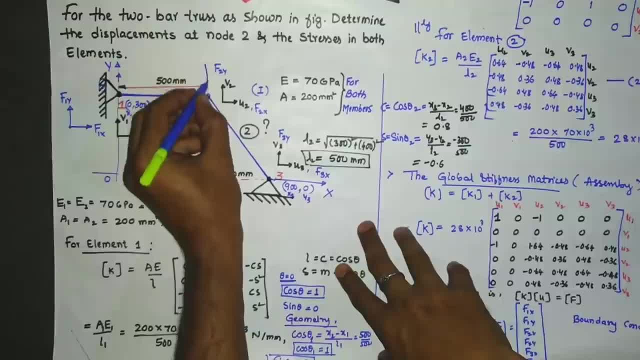 force is applying at. so I have not. force is applying at, so I have not mentioned the 4 in the given diagram, but mentioned the 4 in the given diagram. but mentioned the 4 in the given diagram, but the force is acting at node 2 in. 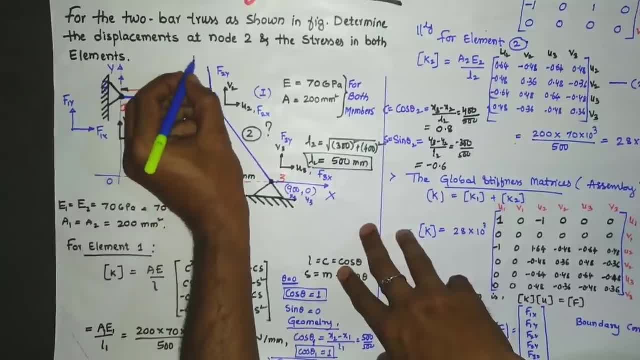 the force is acting at node 2 in. the force is acting at node 2 in downward direction, vertically downward. so downward direction, vertically downward, so downward direction, vertically downward. so that load is 12,000 is given in the, that load is 12,000 is given in the. 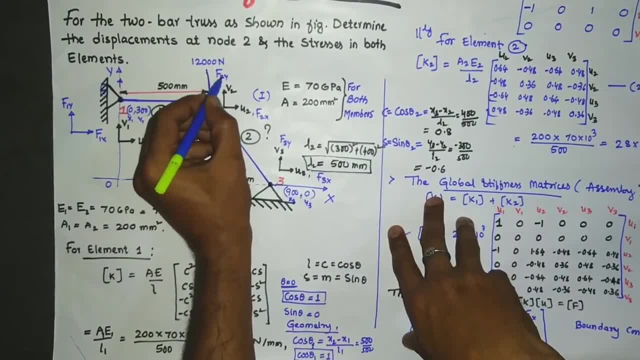 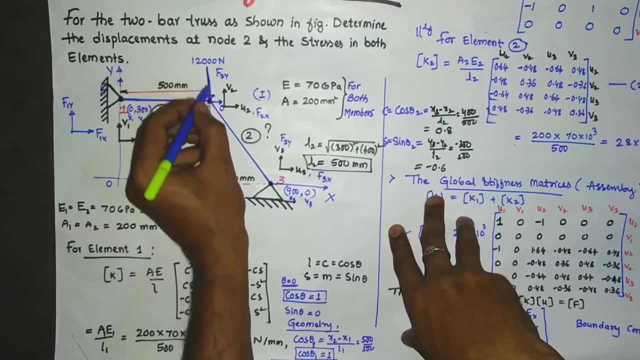 that load is 12,000 is given in the question. so it means that f2y is having question. so it means that f2y is having question. so it means that f2y is having a load and you have to: X is 0 and this. 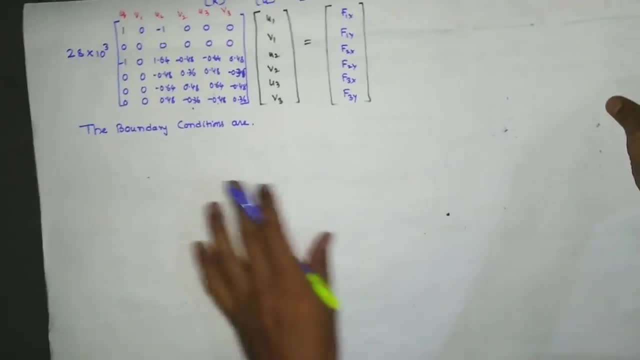 a load and you have to X is 0 and this a load and you have to X is 0 and this is minus or 12,000 after that. so that is minus or 12,000 after that. so that is minus or 12,000 after that. so that boundary condition we have to write so: 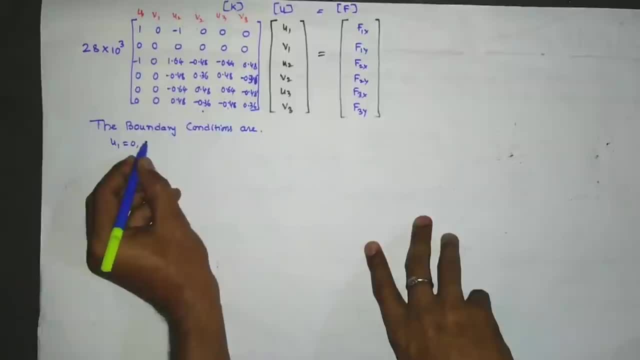 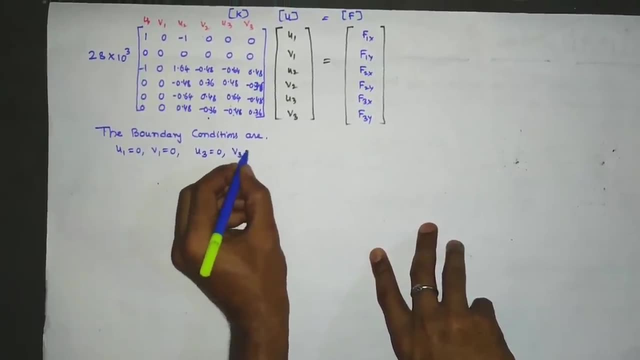 boundary condition. we have to write so: boundary condition. we have to write so: first u1 is equal to 0, v1 is equal to 0. first u1 is equal to 0, v1 is equal to 0. first u1 is equal to 0, v1 is equal to 0 and also u3 is equal to 0, v3 is equal. 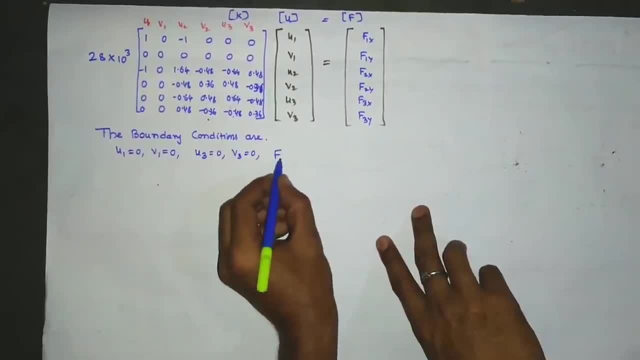 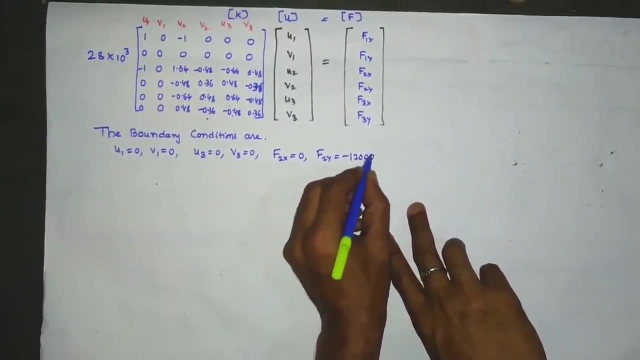 and also u3 is equal to 0, v3 is equal and also u3 is equal to 0, v3 is equal to 0. and now the forces are: you have to X to 0. and now the forces are: you have to X to 0. and now the forces are: you have to X is 0, f2y is minus 12 housing, so we will. 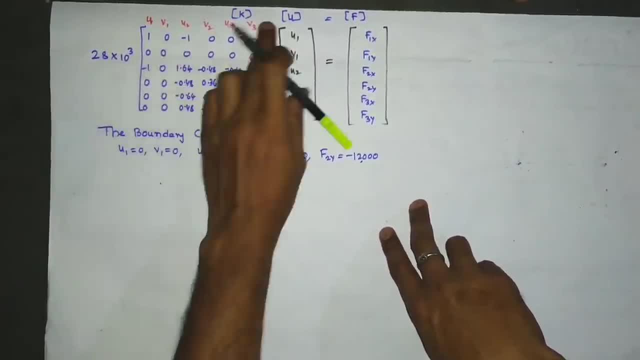 is 0 f2y is minus 12 housing, so we will. is 0 f2y is minus 12 housing, so we will apply these boundary conditions in the. apply these boundary conditions in the. apply these boundary conditions in the formation. so once again, we have to write. 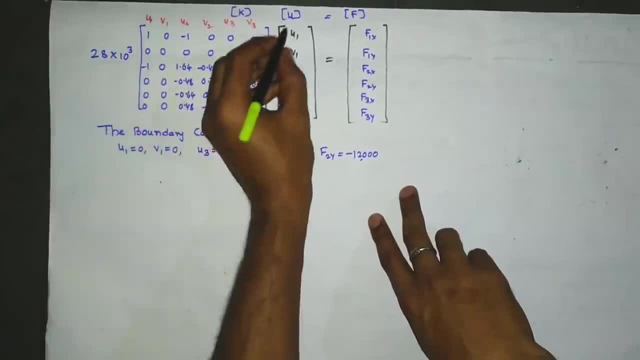 formation. so once again we have to write formation. so once again we have to write the same step here. then we will apply the same step here. then we will apply the same step here, then we will apply this boundary condition. so I am just this boundary condition. so I am just. 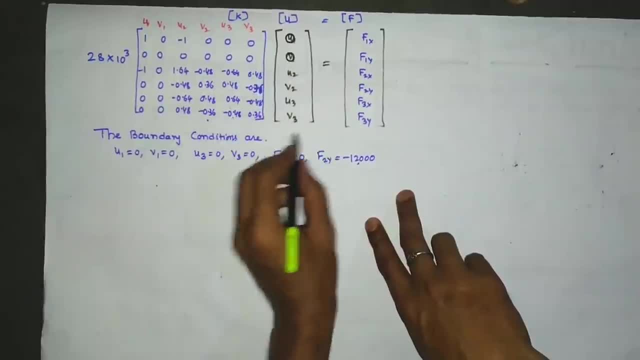 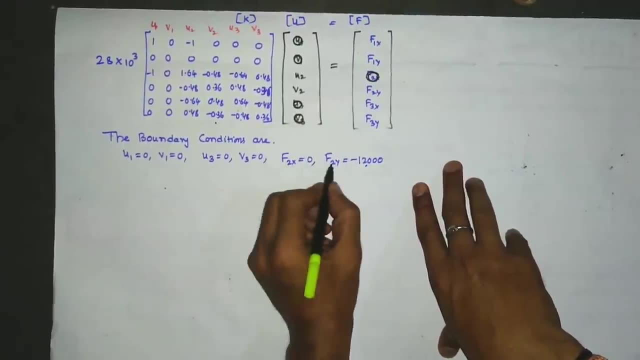 this boundary condition. so I am just making 0: 0 and this is 0: 0 and you have making 0: 0 and this is 0: 0 and you have making 0: 0 and this is 0: 0 and you have to. X is 0, you have to y. 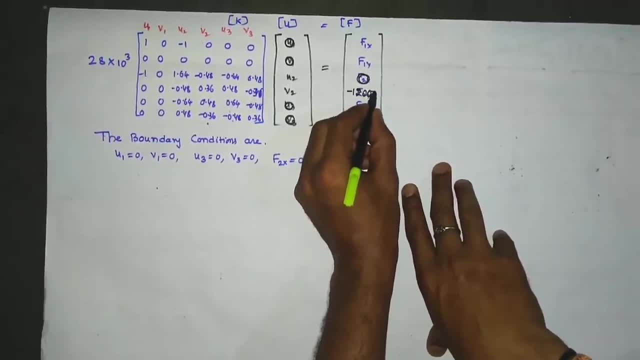 to x is 0. you have to y to x is 0. you have to y is minus 12,000. okay, so 12 will take is minus 12,000. okay, so 12 will take is minus 12,000. okay, so 12 will take 910 power of 3. it will be outside. so this: 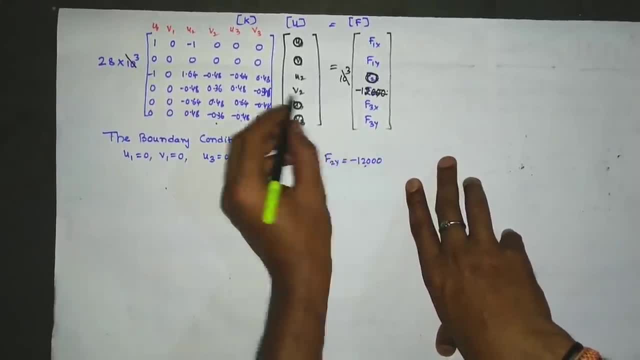 910 power of 3, it will be outside. so this 910 power of 3, it will be outside. so this one, this one will get cancelled. okay, one, this one will get cancelled. okay, one, this one, this one will get cancelled. okay. so after that, the first row, because 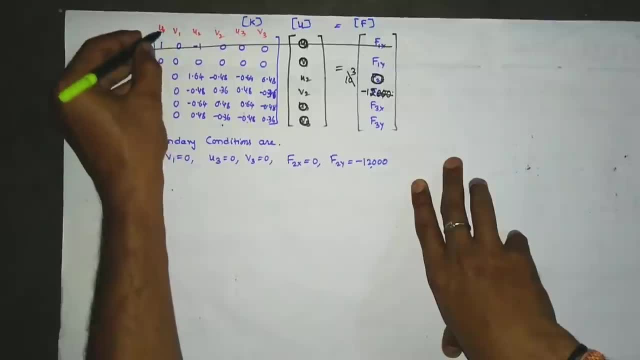 so after that, the first row because. so after that, the first row because of displacement is 0, so their first row of displacement is 0. so their first row of displacement is 0. so their first row and their column it will get cancelled and their column it will get cancelled. 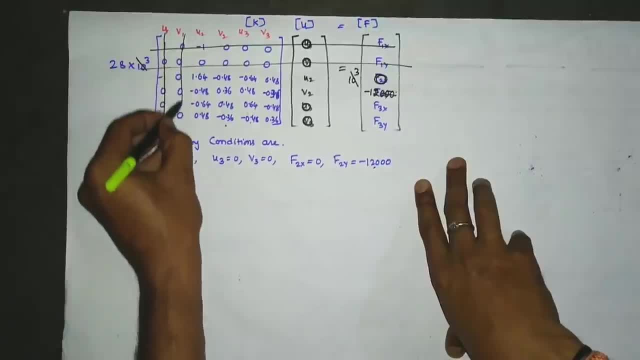 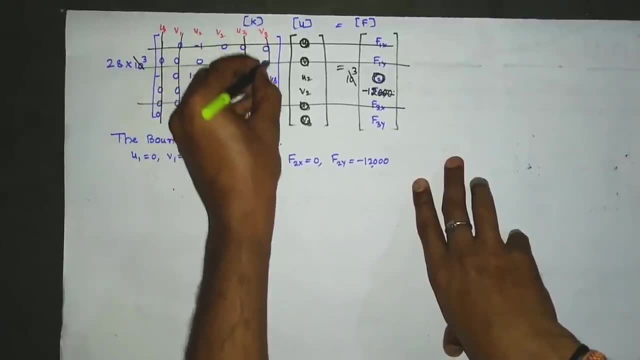 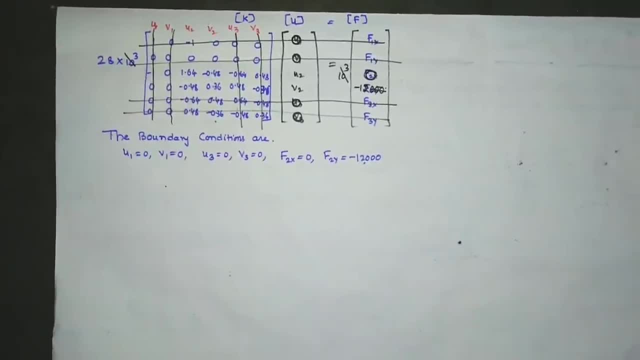 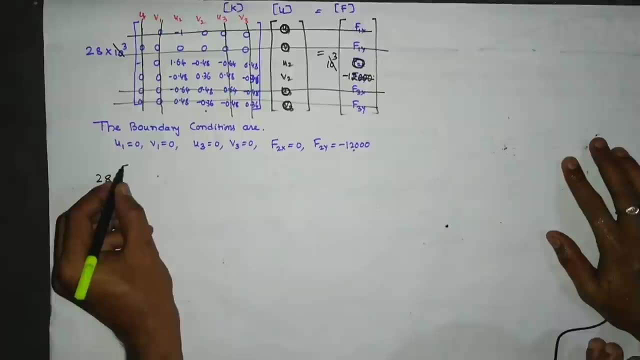 fifth row, fifth column, 6 through 6 column. so after the elimination we will column. so after the elimination we will column. so after the elimination we will have 28 outside and in the matrix. so the have 28 outside and in the matrix. so the have 28 outside and in the matrix. so the remaining value is this: is the remaining. 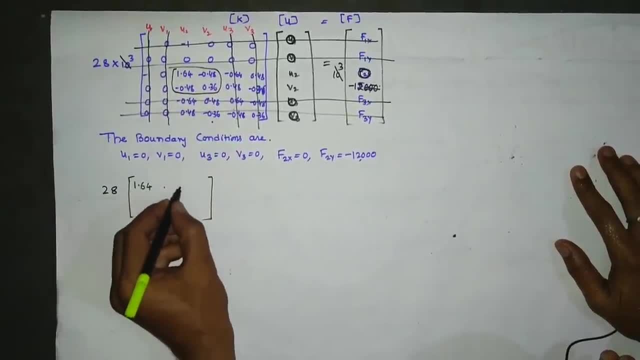 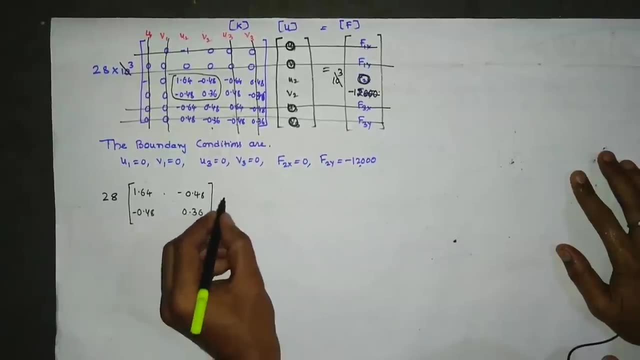 remaining value is: this is the remaining remaining value is: this is the remaining value: 1.64 minus 0.48 minus 0.48 point value: 1.64 minus 0.48 minus 0.48 point value: 1.64 minus 0.48 minus 0.48 point three six: 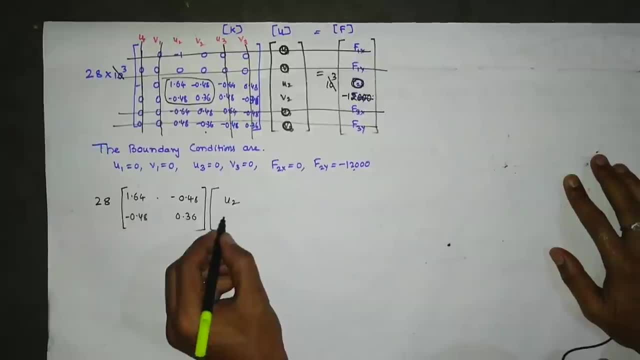 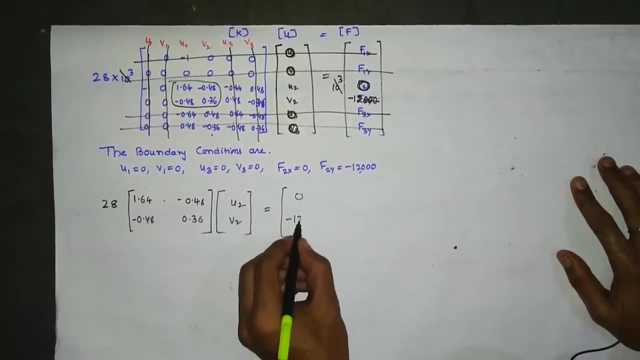 three, six, three, six. into the displacement matrix u2, b2 with. into the displacement matrix u2, b2 with. into the displacement matrix u2, b2 with. the remaining is equal to force vector. the remaining is equal to force vector. the remaining is equal to force vector. that is 0 minus 12. so now, if you make the 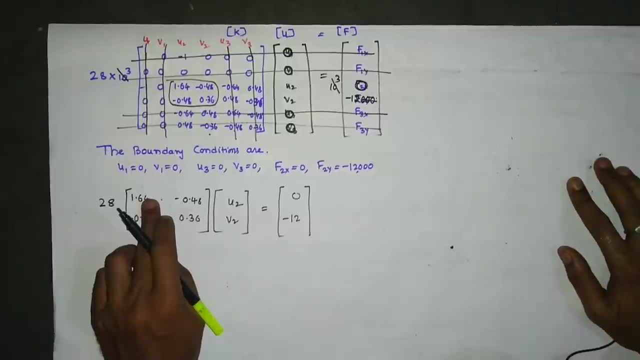 that is 0 minus 12. so now, if you make the, that is 0 minus 12. so now, if you make the multiplication, first take 28 inside the multiplication, first take 28 inside the multiplication, first take 28 inside the matrix. so make the multiplication then. 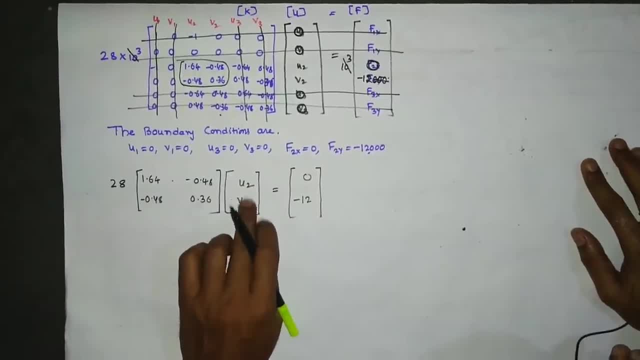 matrix, so make the multiplication, then matrix, so make the multiplication, then after that this matrix it will be. after that this matrix, it will be. after that, this matrix, it will be multiple with a displacement vector is multiple with a displacement vector is multiple with a displacement vector is equal to this two equation. so like that. 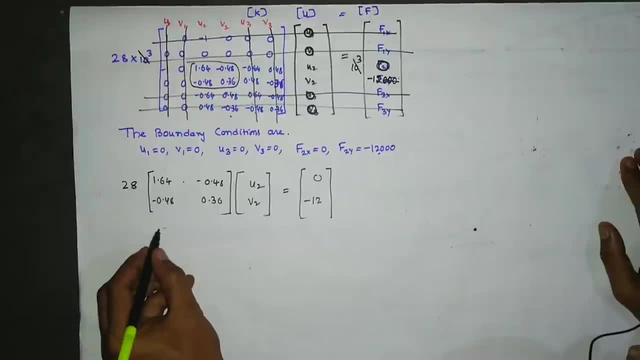 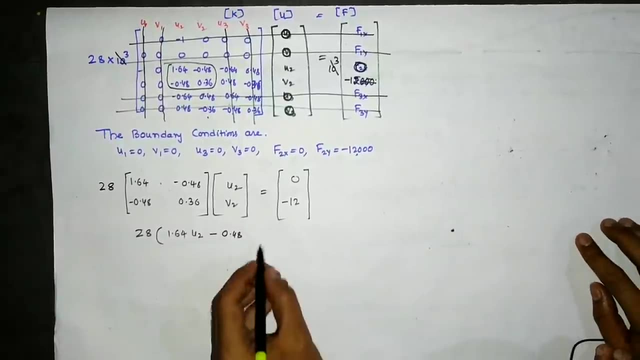 equal to this two equation. so like that. equal to this two equation. so like that. if i made the multiplication, so we will. if i made the multiplication, so we will. if i made the multiplication, so we will obtain 28 outside 0.48. b2 is equal to 0. similarly, 28. 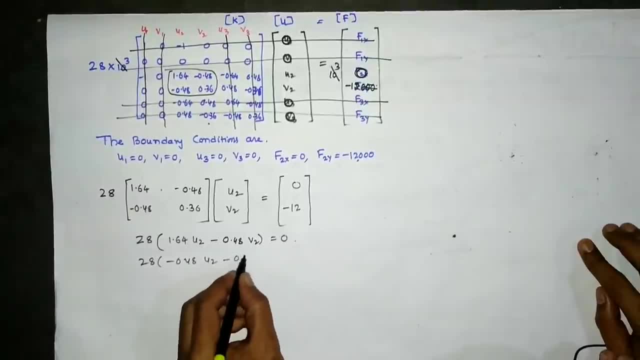 0.48 b2 is equal to 0. similarly, 28: 0.48 b2 is equal to 0. similarly, 28 minus 0.48 u2 minus 0.36 minus 0.48 u2 minus 0.36. 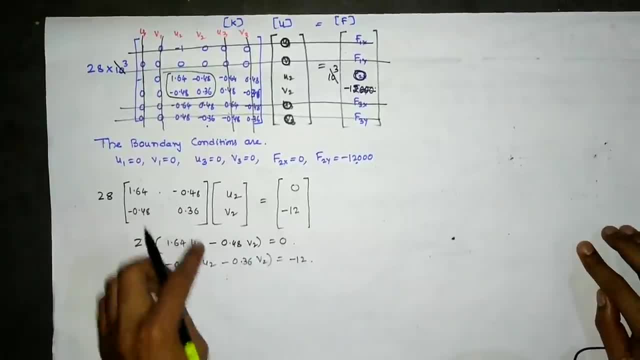 minus 0.48 u2 minus 0.36 b2 is equal to minus 2n. so from these b2 is equal to minus 2n. so from these b2 is equal to minus 2n. so from these two equations we will obtain the u2. 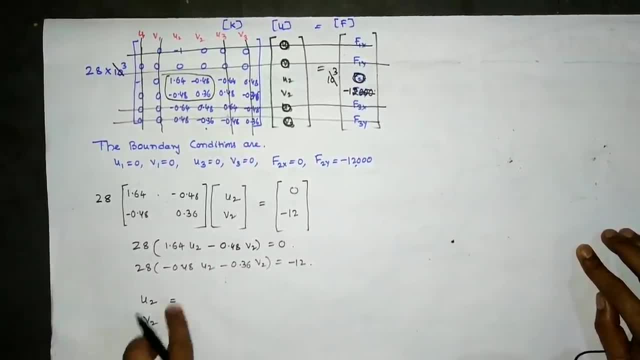 two equations: we will obtain the u2. two equations: we will obtain the u2 value, value value and v2 value, so that value i will write, and v2 value so that value i will write and v2 value so that value i will write directly. so you can make by using the. 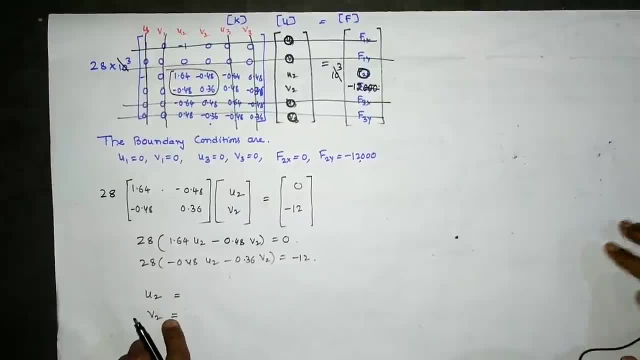 directly. so you can make by using the directly. so you can make by using the calculator, by taking the equation calculator, by taking the equation calculator, by taking the equation, and you will get the u2 v2 value and you will get the u2 v2 value. 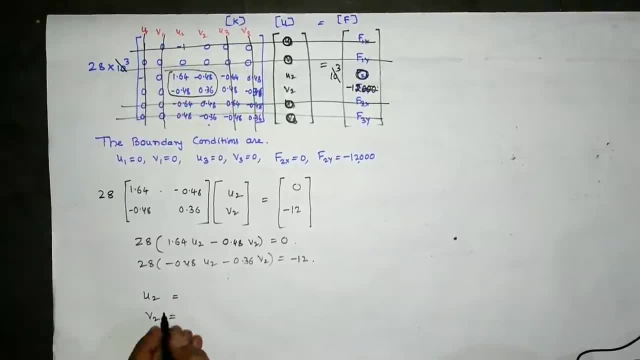 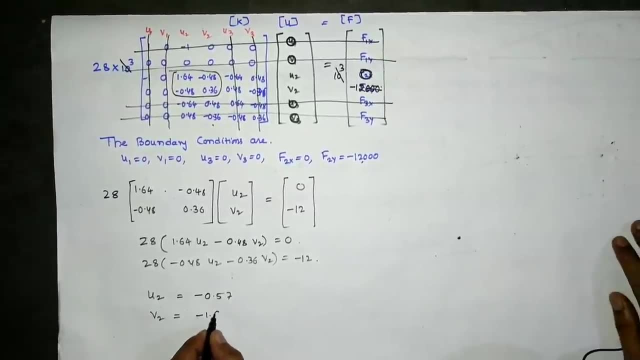 and you will get the u2 v2 value. so from this equation i got, so from this equation i got. so from this equation i got u2 as minus 0.57, u2 as minus 0.57, u2 as minus 0.57 and v2 as 1.96. 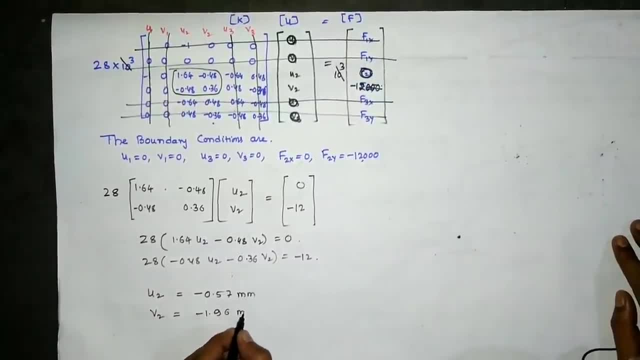 and v2 as 1.96 and v2 as 1.96. so these two values will be millimeters. so so these two values will be millimeters. so so these two values will be millimeters. so these are the displacement, so it unit. these are the displacement, so it unit. 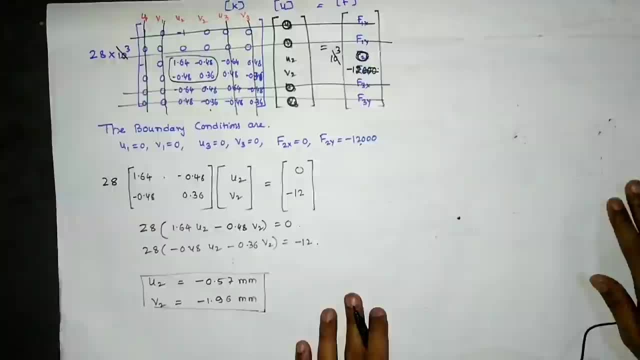 these are the displacement, so it unit will be millimeter, will be millimeter will be millimeter. okay, so after that you need to calculate. okay, so after that you need to calculate. okay, so after that you need to calculate. this in the element that is sigma, this in the element that is sigma. 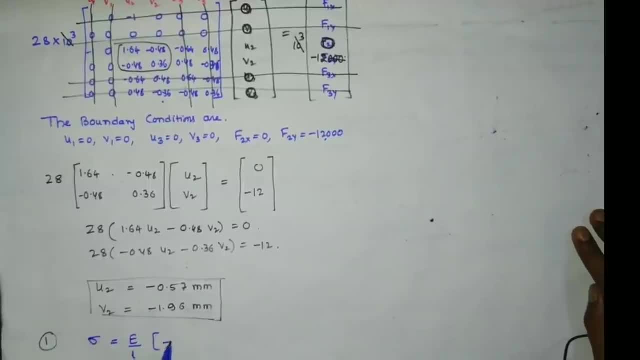 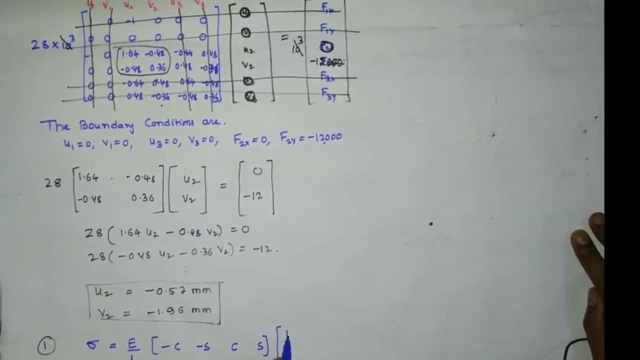 this in the element that is sigma, is equal to e by l, is equal to e by l, is equal to e by l, minus c, minus s, minus c, minus s, minus c, minus s, c, s, c, s, c, s. and here the displacement for the element and here the displacement for the element. 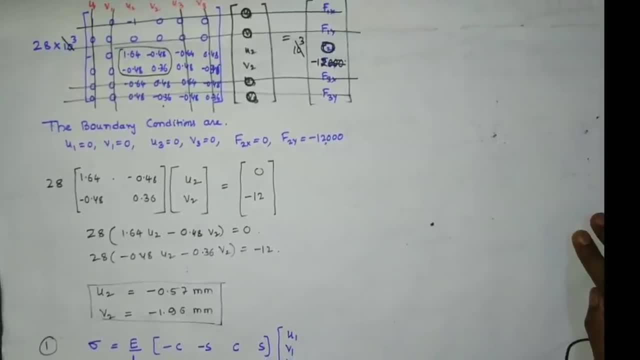 and here the displacement for the element: suppose, if it is element one, suppose, if it is element one, suppose, if it is element one: u1, v1, u2, v2, u1, v1, u2, v2, u1, v2, v2, and here it will be e1, l1 for element one. 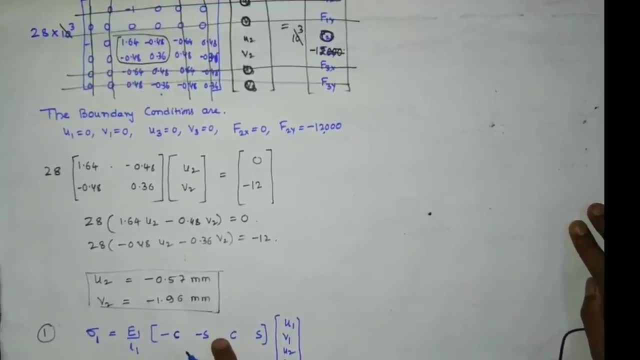 and here it will be e1 l1 for element one, and here it will be e1 l1 for element one. so c value which you have already, so c value which you have already, so c value which you have already calculated for, calculated for, calculated for element one, so that you have to 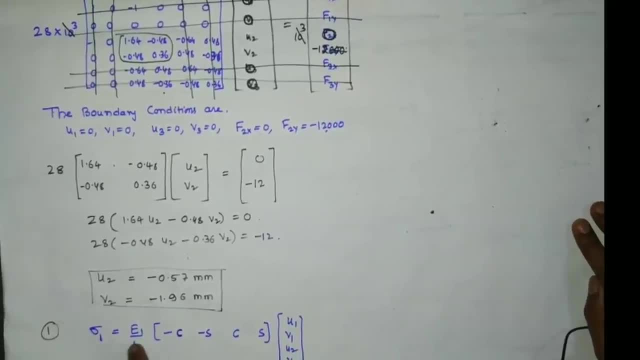 element one so that you have to. element one, so that you have to substitute here, substitute here, substitute here. okay, so so that after the multiplication, okay so so that, after the multiplication, okay, so so that after the multiplication, you will get the, you will get the, you will get the stress in the element. 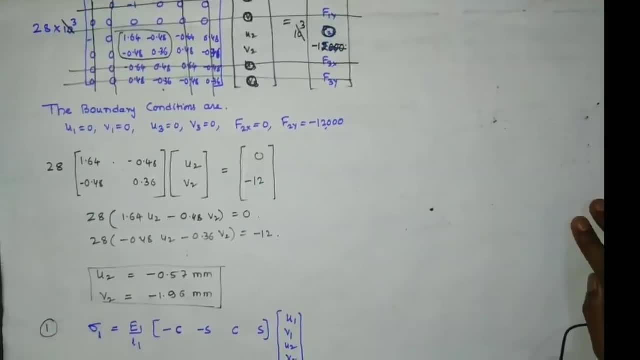 stress in the element, stress in the element. so i will write the direct answer for. so i will write the direct answer for. so i will write the direct answer for this, which i have already calculated, this which i have already calculated, this which i have already calculated, so the stress for the element one, i 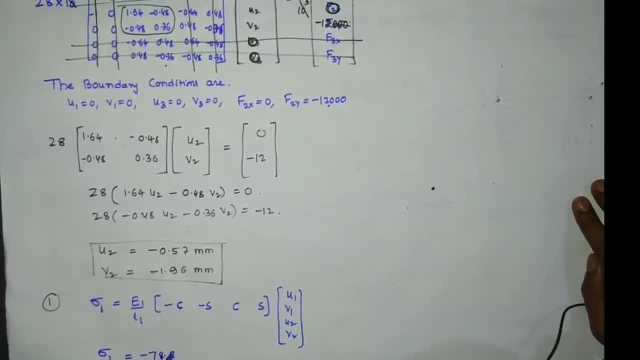 so the stress for the element one: i. so the stress for the element one i. obtained minus 79.8. obtained minus 79.8. obtained minus 79.8 newton per millimeter square 79.8 newton per millimeter square 79.8. 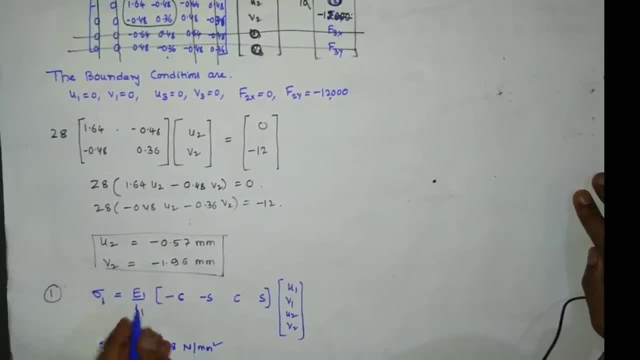 newton per millimeter square 79.8. similarly for element two. similarly for element two. similarly for element two. for element two, it will be e2. for element two, it will be e2. for element two, it will be e2- e2 l2 minus c. 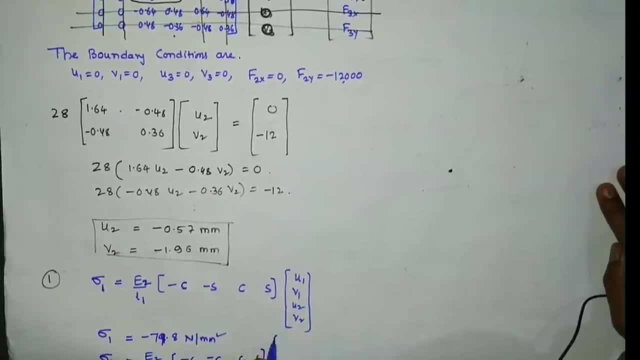 e2 l2 minus c. e2 l2 minus c minus s c s. so here the displacement it minus c minus s c s. so here the displacement it minus c minus s c s. so here the displacement it will be will be: will be u2, v2, u3, v3.